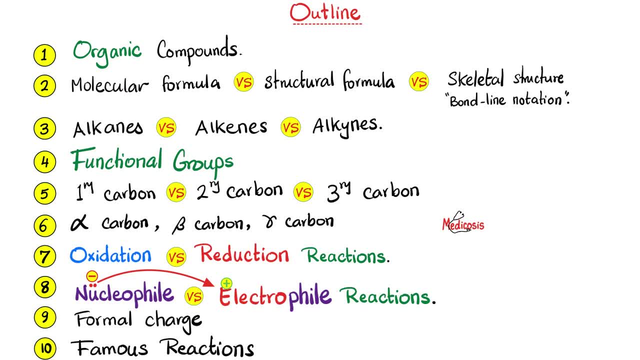 Organic compounds versus inorganic compounds, Molecular formula versus structural formula versus condensed structural formula versus the skeletal structure, the backbone, the bond-like notation, Alkanes versus alkenes versus alkynes. Alkenes have a single bond between carbon and carbon. Alkenes have double. 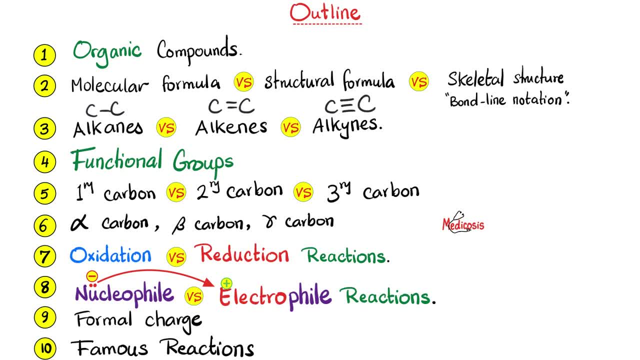 bond between carbon and carbon, And alkynes have triple bond between carbon and carbon. Quick note: the alkanes have single bond. The single bond is the longest, but it's also the longest. How about the double bond? Well, it is shorter than the single bond, but stronger, And as 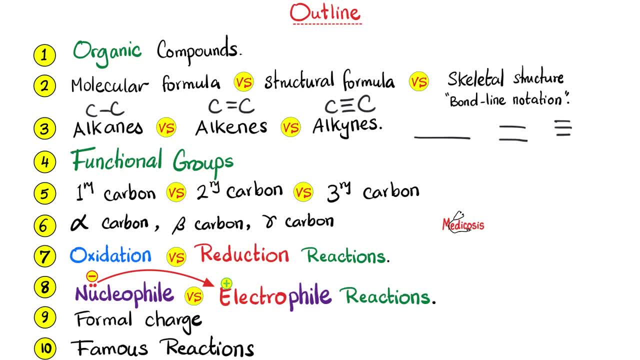 for the triple bond. it is the shortest, but the strongest. Then we'll talk about the famous functional groups, the distinction among primary carbon, secondary carbon, tertiary carbon, quaternary carbon and the distinction among alpha carbon, beta carbon, gamma carbon, etc. 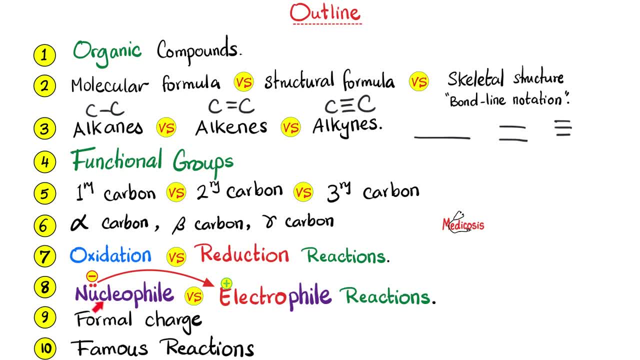 The difference between oxidation and reduction, What's the difference between the nucleophile and the electrophile, And then how to calculate the difference between the nucleophile and the electrophile. What's the difference between the nucleophile and the electrophile, And then how to. 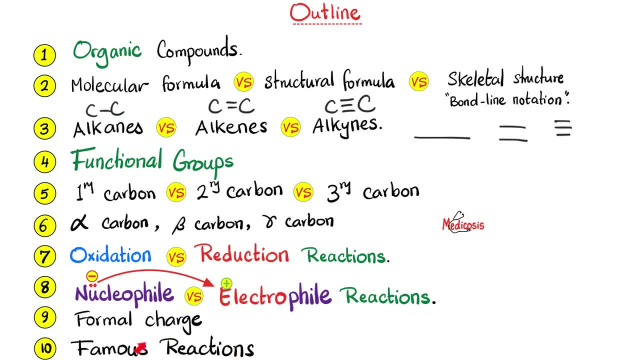 calculate the difference between the nucleophile and the electrophile, And then how to calculate the difference between the nucleophile and the electrophile, And then how to calculate the formal charge, and some famous reactions that you should never miss on your exam, because these are just giveaways. 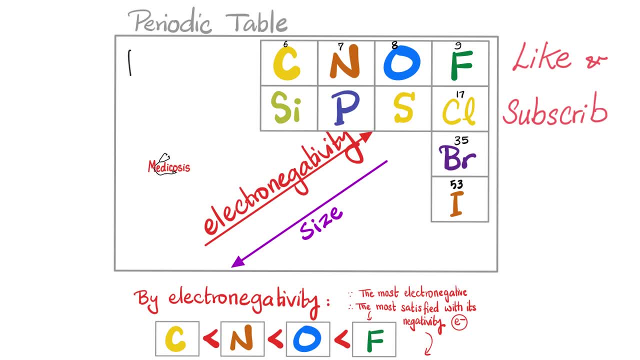 First you need to know the following periodic table elements by heart: First hydrogen, then carbon nitrogen, oxygen, fluorine, silicon, phosphorus, sulfur, chlorine. Under chlorine there is bromine and there is iodine. Electronegativity increases as you go up and to. 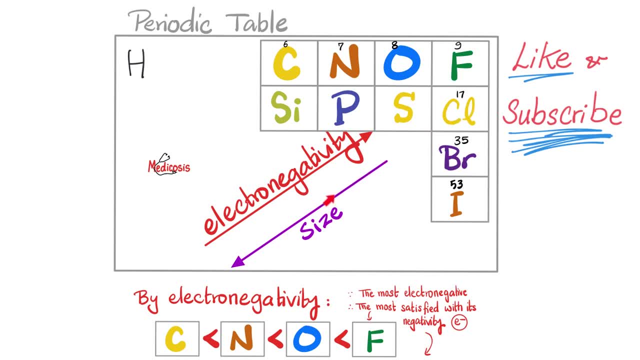 the right, making fluorine the most electronegative. Size increases as you go down and to the left. Fluorine is bigger than flu, Boys is bigger than chlorine and iodine is bigger than bromine. What do you mean by saying that fluorine is the most electronegative? It means 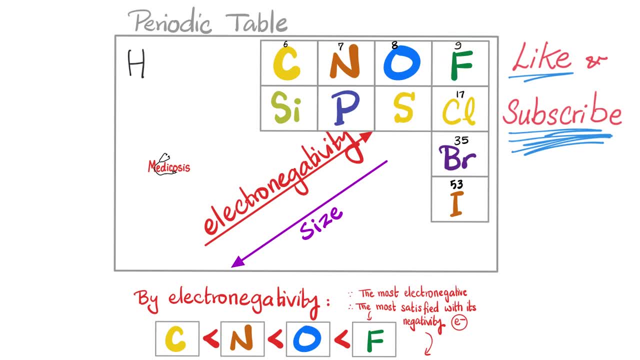 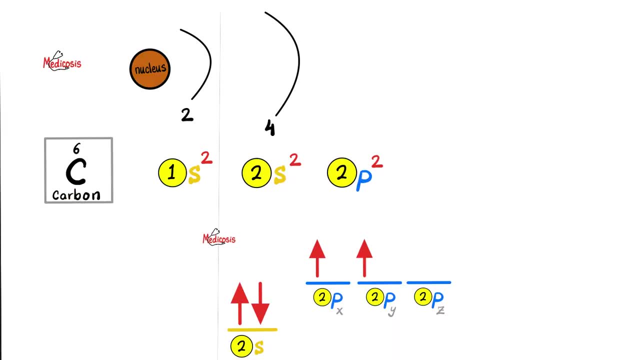 that fluorine is happy and satisfied by the surrounding negative electrons. It is happy with its own negativity. Organic chemistry is the chemistry of carbon. Carbon is element number six in the periodic table, meaning it has six electrons in total, the first two electrons and the first electron. shall I said, shall not. 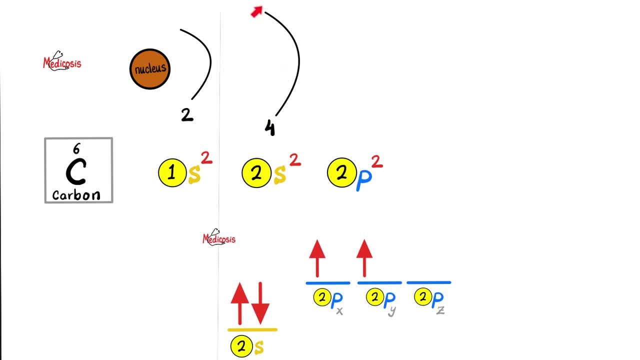 sub-shell And then the last four electrons will be in the valence electron shell. The two electrons here are in 1s2 sub-shell. As of these four electrons, they are 2s2 and then 2p2.. Two in 2s. 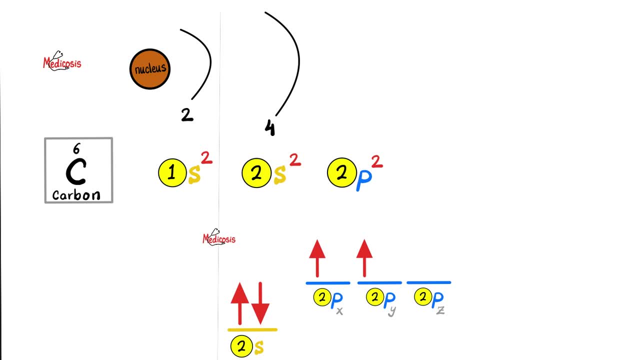 and two electrons in 2p. If you want to draw 1s2, you can draw it like this, with two electrons with opposite spin, but then you ignore this. in organic chemistry We'll focus on these and that will be a huge topic coming later, which is sp3 hybridization versus sp2, hybridization versus sp. 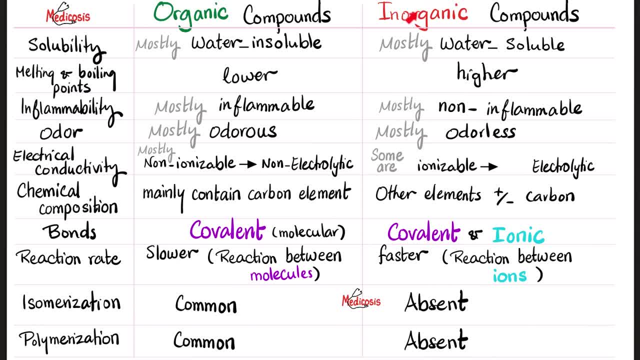 hybridization. Let's compare between organic compounds and inorganic compounds. Solubility: Organic compounds are mostly water-insoluble. Who's gonna dissolve them then? Something organic just like them, For example benzene. As for inorganic compounds, they are mostly water-soluble. 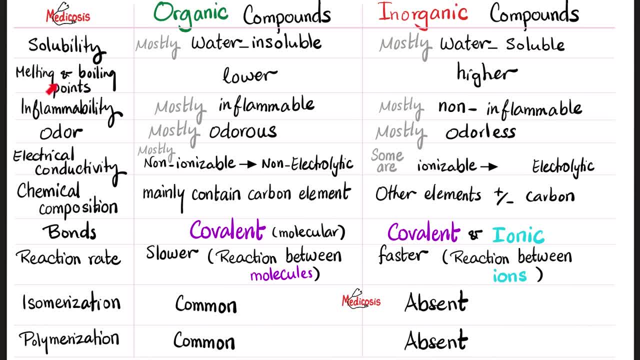 Think of sodium chloride, for instance. Boiling points In melting points. relatively speaking, organic compounds have lower melting points or boiling points compared to their inorganic counterparts. Inflammability: Organic compounds are mostly inflammable, but inorganic mostly non-inflammable. Odor: Organic compounds have lovely odors. 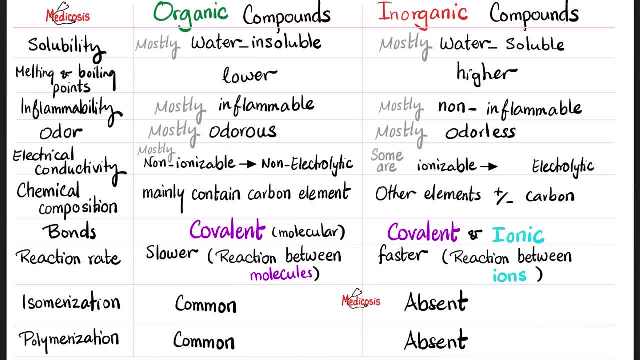 many of them- vanilla, cinnamon and others- are indeed organic compounds. And why do you think the aromatic? organic compounds are called aromatic? Because they are smelly. They have distinctive scents, So inorganic compounds are mostly non-inflammable. So inorganic compounds are. 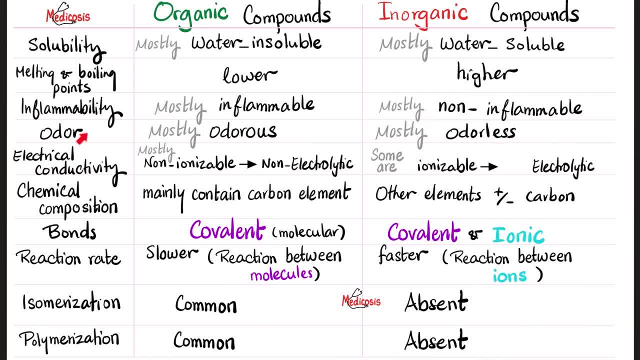 odors, Inorganic ones, mostly odorless. Electrical conductivity: Organic compounds are mostly non-ionizable and that's why they are non-electrolytic. But inorganic compounds- many- are ionizable and therefore electrolytic. Again, think of something half positive like this and half 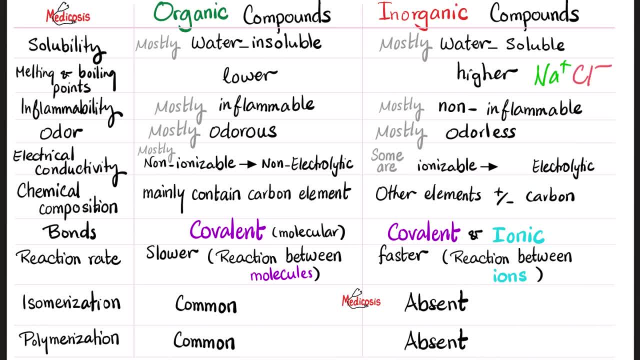 negative. Is this ionizable Yup electrolytic? Some are more electrolytic than others, of course. Chemical composition: Organic compounds are mainly made of carbon elements. Inorganic other elements, let's say I have sodium, I have chlorine, iodine, magnesium, potassium. 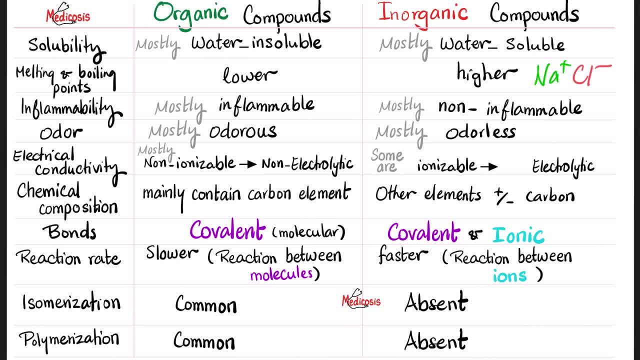 and sometimes carbon. Chemical bonds, Organic compounds, covalent, or molecular bonds: Inorganic could be covalent, could be ionic Reaction rates. Since the reactions here are happening between molecules, they are slower, But here the reactions are mostly between ions. so 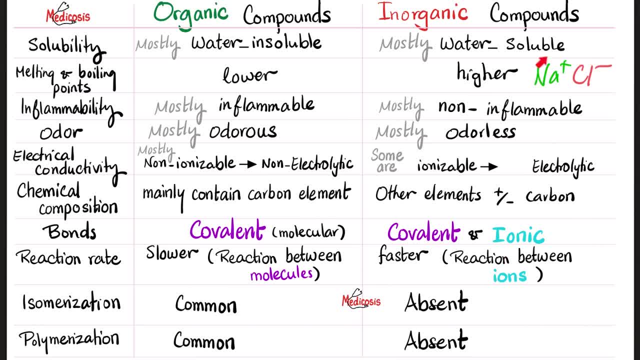 they are faster. These ions can dissociate very quickly and react very quickly. Isomerization is very common in organic Inorganic compounds. We do not see it for the most part, Polymerization. Organic compounds do make polymers, Inorganic compounds do not. What does poly mean? It means many And mere 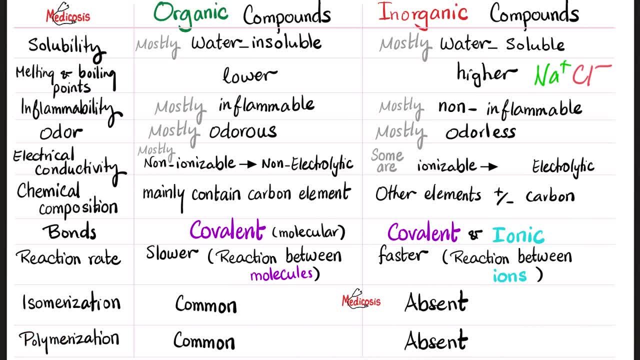 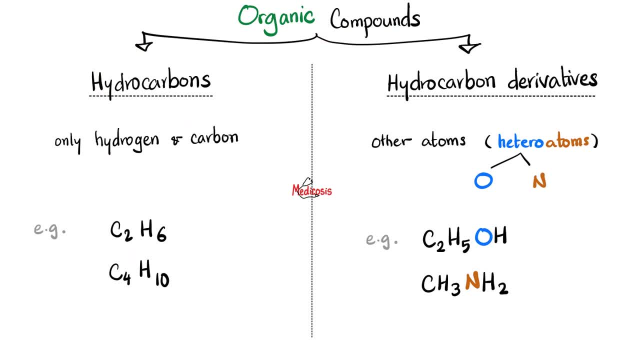 means piece, So many pieces bound to one another. Plastic is one example. Organic compounds or carbon land could be hydrocarbons, which means only hydrogens and carbons. just like this, For example: here are two carbons and then we have six hydrogens. just like this. 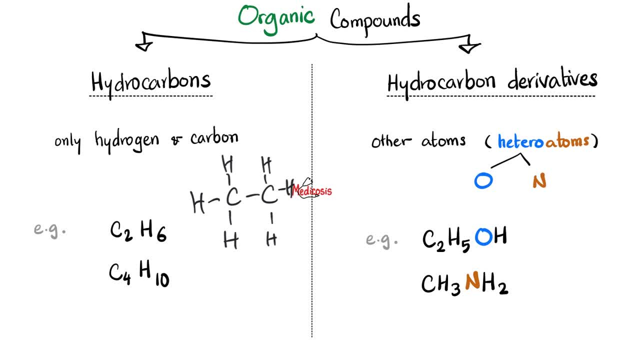 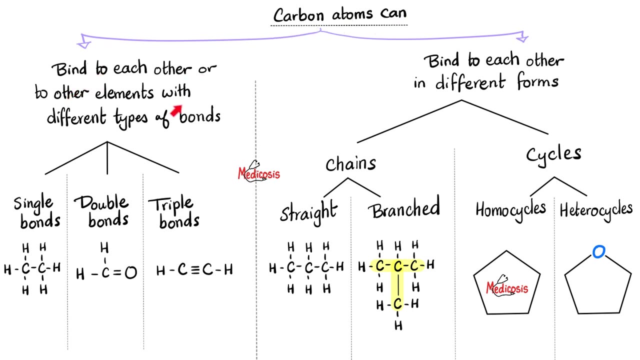 hydrocarbon, because I only have hydrogens and carbons, But I could have other atoms called heteroatoms, something else besides hydrogen and carbon. This could be oxygen or could be nitrogen. Carbon is so versatile. Why? Because carbon atoms can bind to one another or to other elements with. 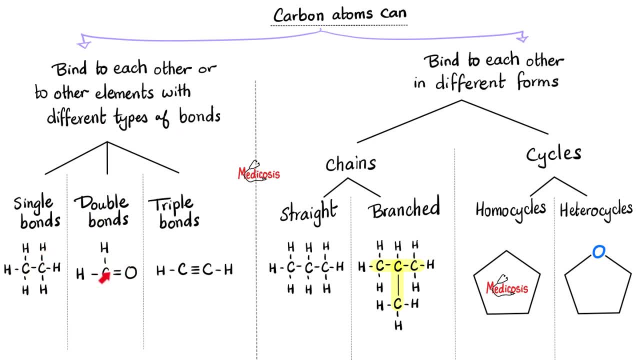 different types of bonds. Could be single bonds, could be double bonds, like this one, or could be triple bonds, just like this one. Carbon atoms can also bind to each other in different forms, such as a chain or a cycle. The chain could be a straight chain. Look at the carbons here. straight chain. 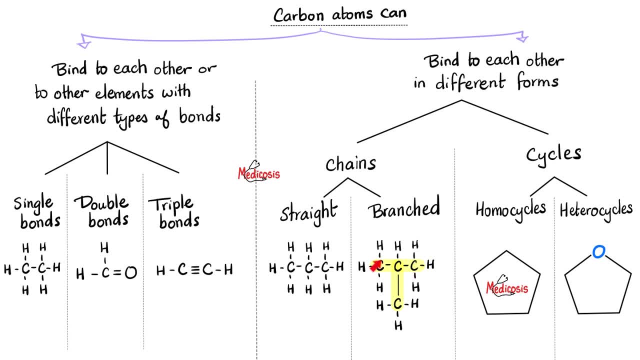 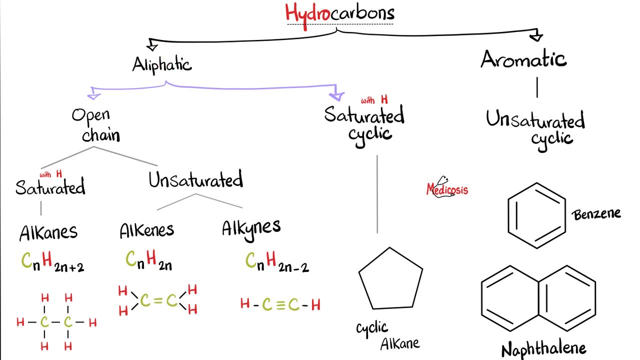 How about branched? Oh, look at this, here's a straight chain, but I have a branch. Now, if you have watched my biochemistry videos, can you remind me what were the branched chain amino acids? Let me know down below in the comments. Hydrocarbons, hydrogens and carbons could be aliphatic. 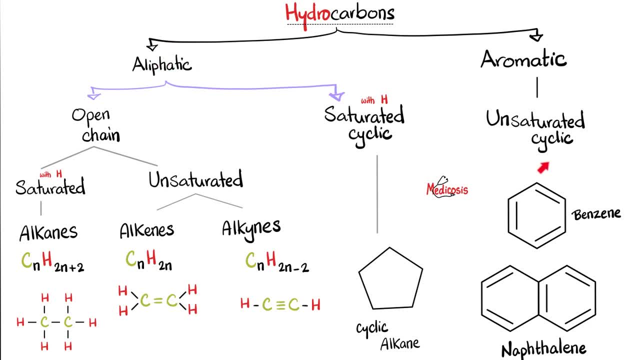 which means no benzene ring, or aromatic, which means we do have benzene rings. The aliphatic could be an open chain, just like this, or saturated cyclic, just like this. What do you mean by saturated? I mean saturated with hydrogen. There is nothing but carbon-carbon single bonds and 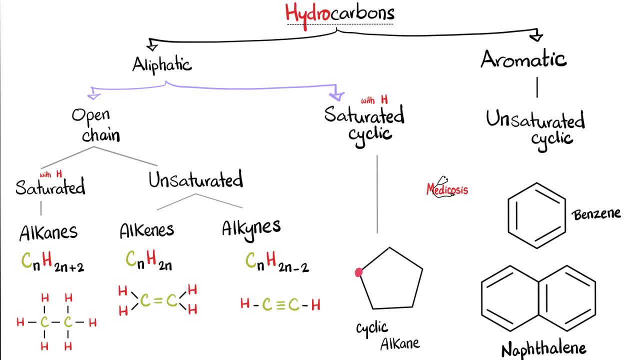 hydrogens. So here is a bond between one carbon and the next carbon, and then the rest is two hydrogens here and I have two hydrogens there. Why two? Because carbon makes four bonds in total. So for this carbon atom here's one, two, three and four. 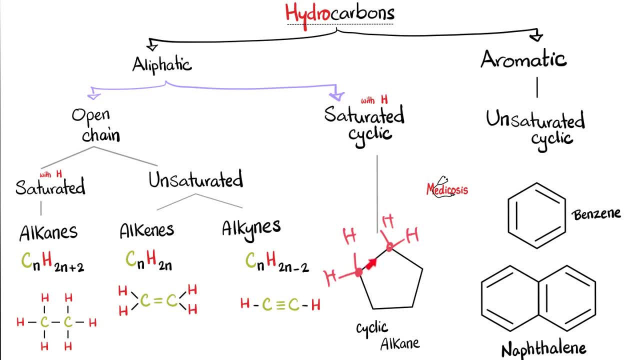 bonds For this carbon atom. here's one, two, three and four bonds, And the same thing for the rest of this, and this is a cyclic alkane. How many carbons? One, two, three, four and five. This is cyclopentane. 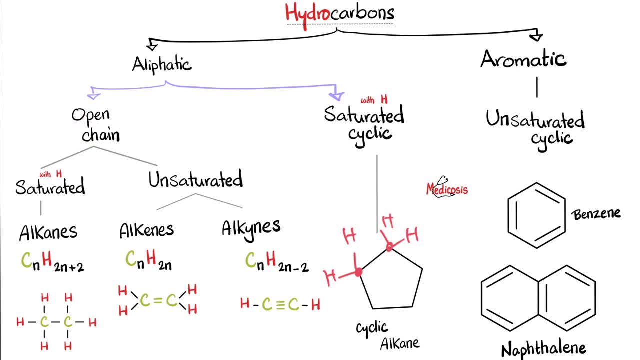 because penta means five. As for the aliphatic open chain, they could be saturated Whenever you hear of saturated with hydrogen, which means I have nothing else but single bonds between carbons and the rest is hydrogen. How about unsaturated? They have less hydrogen than they can Look at. 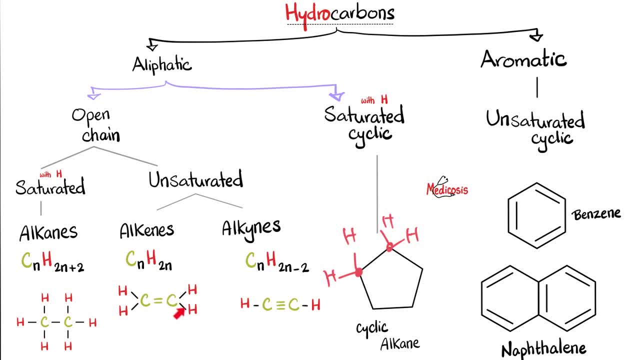 this. This carbon is connected with three hydrogens. but look at this carbon: It's connected with only two hydrogens because I gotta preserve one for my double bond. So it has less hydrogen than this. If you have less hydrogen, you're unsaturated with hydrogen, But if you're saturated, 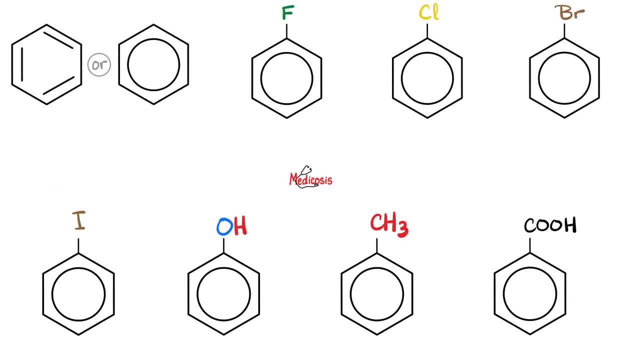 you're saturated with hydrogen to the fullest. Can you name these lovely compounds? Let's try this. The first one is the benzene, and you can draw it like this, or you can draw it like this: Notice that it ends in "-ene", just like alkene, which reminds me of the double bonds. Is this aliphatic? 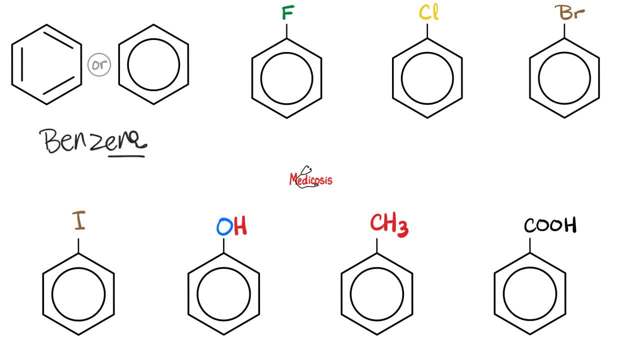 or aromatic? Of course, aromatic. How about this one fluorobenzene and this chlorobenzene, This one bromobenzene, This one iodobenzene And this one chlorobenzene And this one chlorobenzene And this one? 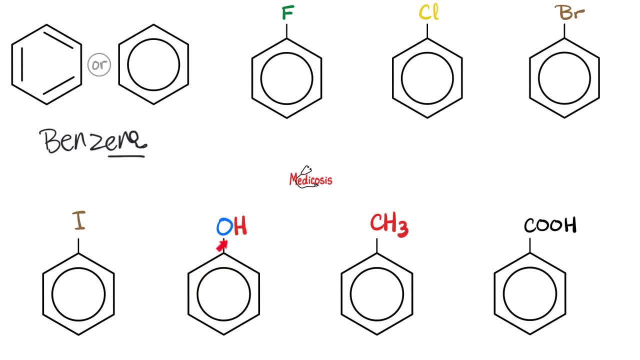 you can call it hydroxybenzene, or better phenol. How about this? methylbenzene, or better toluene? And this, remember, COOH? This is a carboxylic acid group, Carboxylic acid plus. 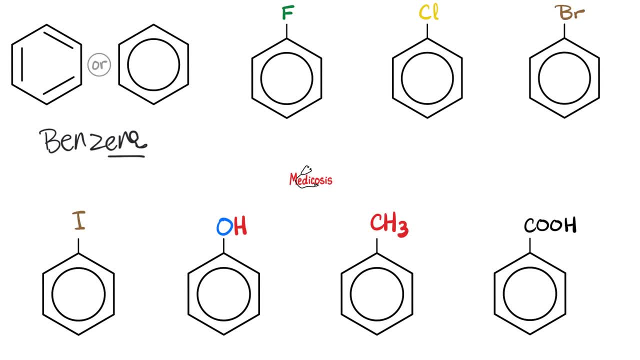 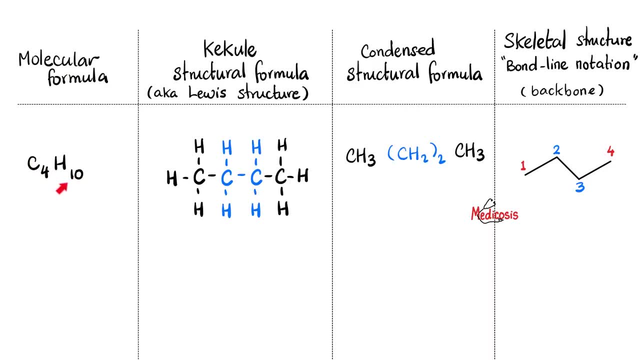 benzene. together is benzoic acid. And here are the names. Please pause and review. Here is the molecular formula: Four carbons, ten hydrogens, C4H10.. If you break this down, this is carbon and this is hydroxybenzene And this is hydroxybenzene And this is hydroxybenzene And this is. 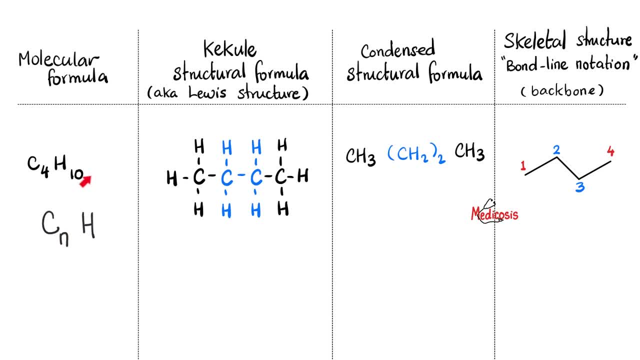 hydrogen. Suppose that 4 is the N and therefore the relationship is: N is 4.. 2N will be 8.. 2N plus 2 will be 10.. Just like that, When your formula is CnH2N plus 2, this is an alkane, All of them. 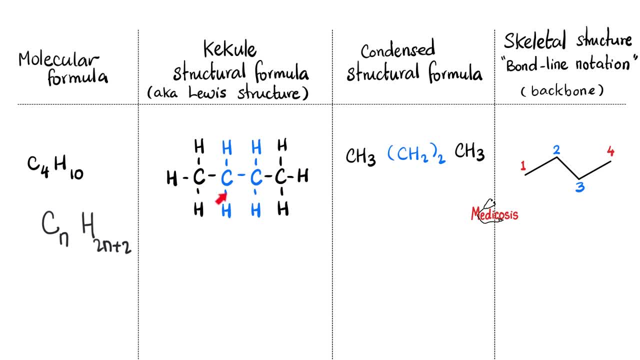 are single bonds, as you see here. So can I open this up? Yes, And this is called Kekul structural formula or Lewis structure. Of course, lovely scientists always argue with one another about who discovers which is which, So let's start with this. Let's start with this, Let's start with this. 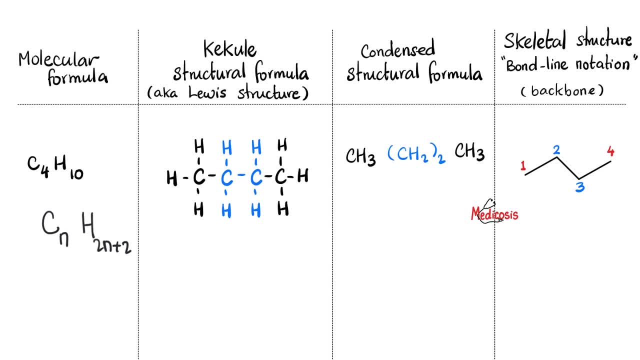 Who discovered this formula first, One of the oldest tricks in the book. I don't know what I'm talking about. Condensed structure formula is more condensed than this. So let's make this CH3. And then I have CH2, and then CH2 again, So it's CH2 times 2.. And then the last one is CH3. This is 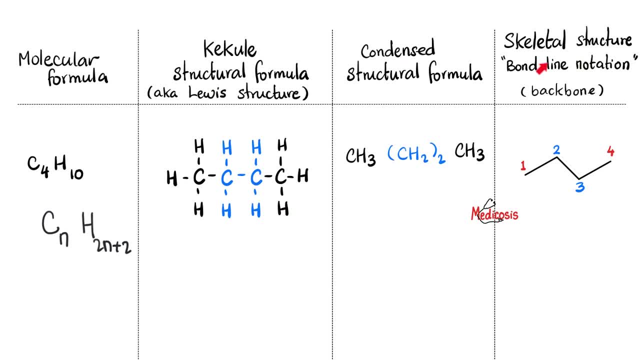 called condensed structural formula. Okay, The last one is the skeletal structure or the bond line notation. Since this is hydrocarbon and hydrocarbons are always implied, we can just do lines like this like a backbone of hydrocarbons. Each one of this is a carbon, So here's one. 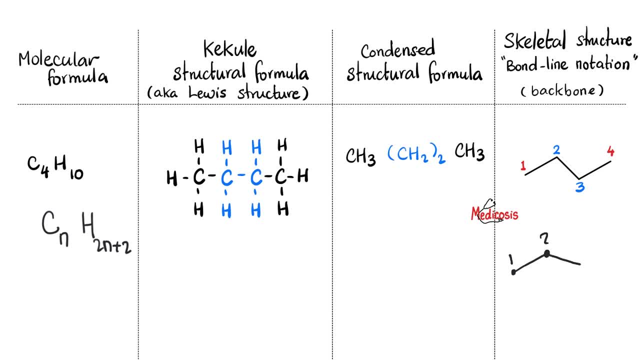 carbon. Here's the second carbon. when you stop And then you go down like this, This becomes the third carbon. And you go up like this, This becomes the fourth carbon. You do not have to draw the dots, I'm just trying to help you understand. where did this come from? So the line is not the carbons. 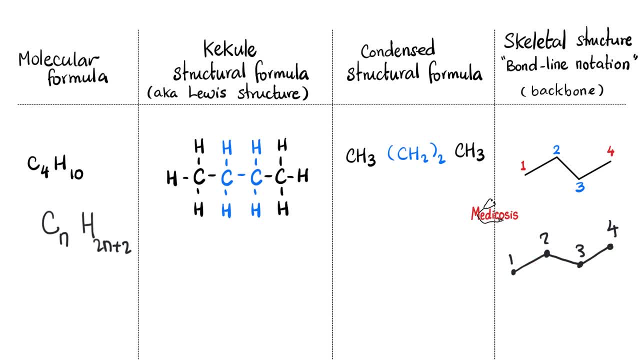 The lines are the covalent bonds, The dots are the carbons. Okay, If the dots are the carbons, where are the hydrons? then? They are hidden, They are implied. So this one will have three hydrogens, just like this, And this one will 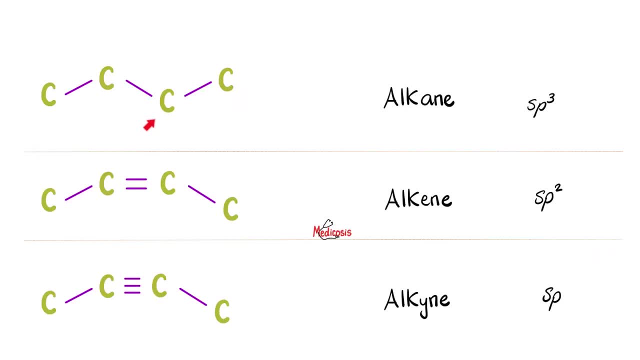 have two hydrogens, two hydrogens, three hydrogens: Alkanes, alkenes and alkynes. Let's focus on this. carbon. Here is a bond, Here is a bond. Carbon makes four. So here is three and here is four. 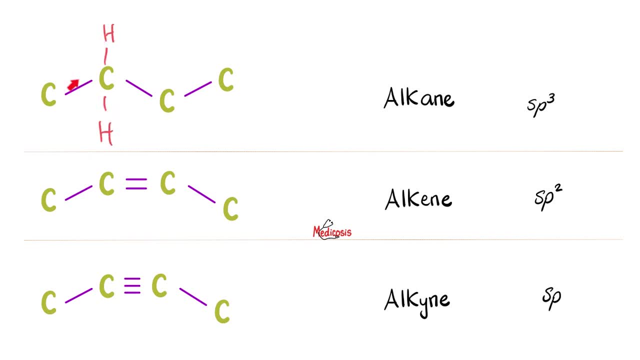 Amazing, How many do you have? I have four groups: One, two, three and four. So you draw what you saw like this: Three dashes S, times, P, times P. Multiply them together, You get S P to the third. 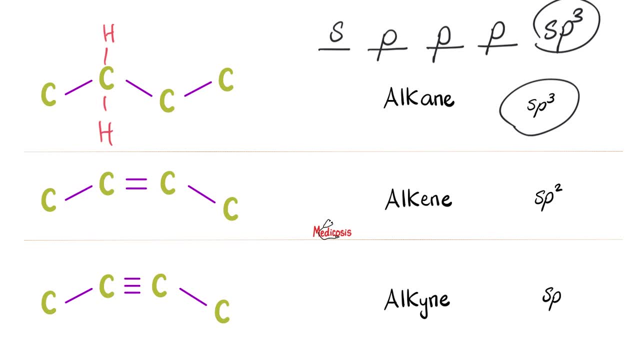 power or sp3 hybridized. But try your luck here. Look at this carbon. Here is one bond, second bond, third bond, which means there is a hydrogen hidden here. Let's count the groups: Here is one group, Here is one group And here is one group, So all of them are three. You draw what you saw like this: 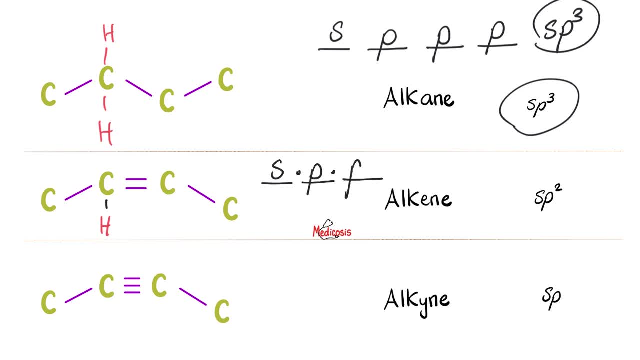 Three dashes S times P, times P. Multiply them together, It is S, P to the second power, or sp2 hybridized. As for this carbon, I have one bond, two bond, three bond, four bonds, which means there are no hydrogens here. How many groups? Here is the. 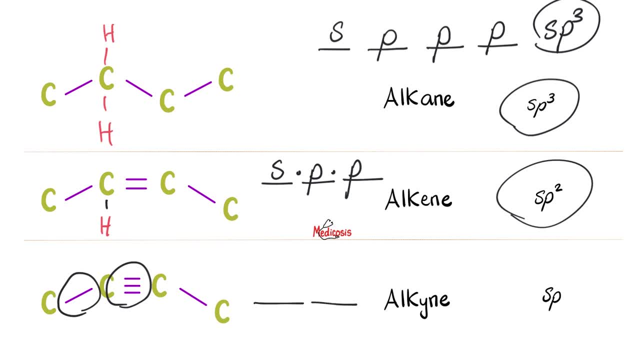 first group. Here is the second group. Draw what you saw. Two groups S times P is sp hybridized, and this is the easiest trick to remember them on your exam. Why are these like? this is another topic for an upcoming video titled sp hybridization. 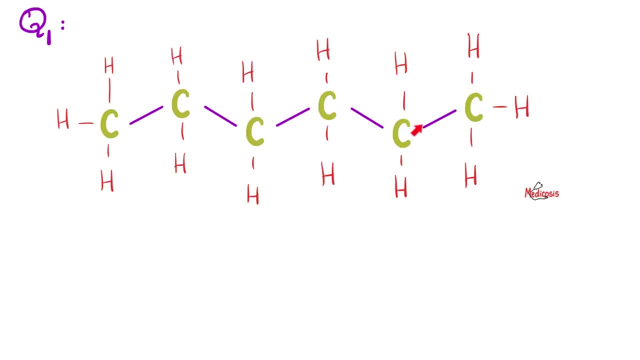 What's the name of this? Well, 1,, 2,, 3,, 4,, 5,, 6.. All of them are single bonds. This is a hexane, which is a type of alkane. How about this? 1,, 2,, 3,, 4,, 5, 6.. Hydrogens are hidden, It's the same. 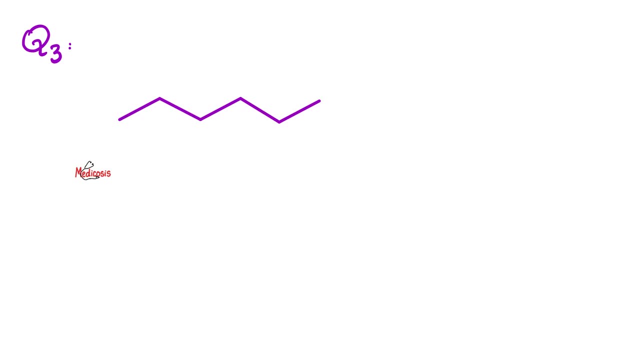 molecule. It is also hexane. And this, Here's the first carbon. Here is the second carbon. Here's the third carbon. Here's the fourth carbon, fifth and sixth carbon. Guess what? It's the same hexane. 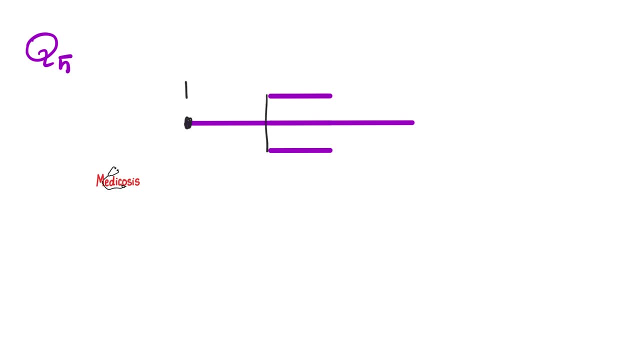 How about this? This weird thing right here? Here is my first carbon. This is a triple bond. So this is second carbon, third carbon and fourth carbon. How many carbons do you have? You have four. The word for four in organic chemistry is butane, And since you have a triple bond between two and three, 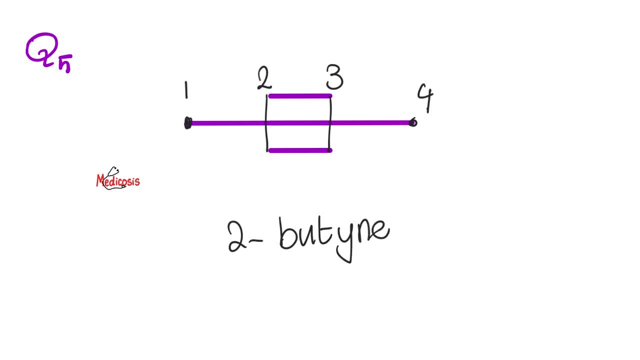 it is butane And two and three. which one is the lowest number? The lower is two. So you write two butane To emphasize that the triple bond is between the second carbon and the third carbon. We will learn more about this in the next video. 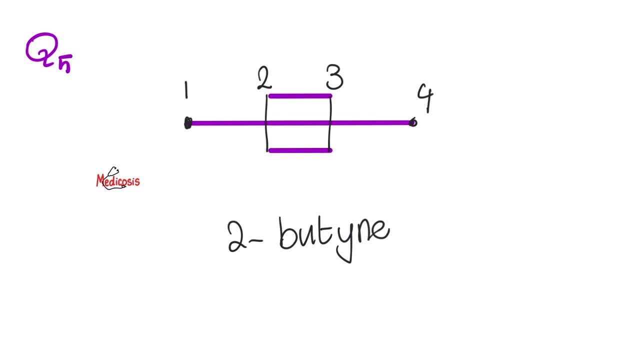 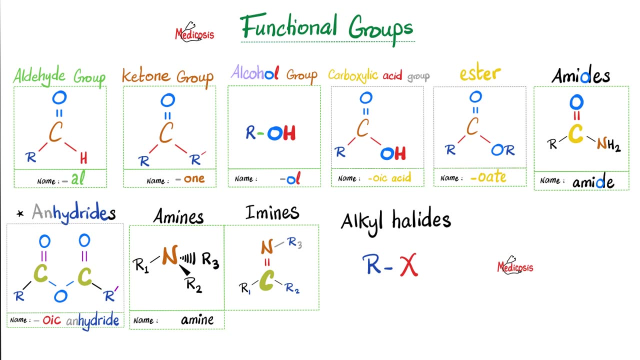 The famous functional groups for your exam. First, remember your water, which is H-O-H. Remove this H, replace it with a hydrocarbon chain or the rest of the chain, whatever that is, and you get an alcohol group. Modify this into C-O-O-H, That's a carboxylic acid. 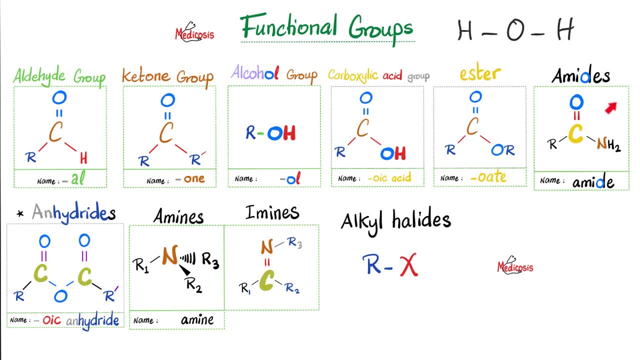 What are the derivatives of the carboxylic acids? Esters, amides, anhydrides. What's the aldehyde? C-O-H or C-H-O, Ketone groups, C-O. but instead of the H we have another chain, A chain on this side and a chain on that side. Aldehydes end in L, Ketones. 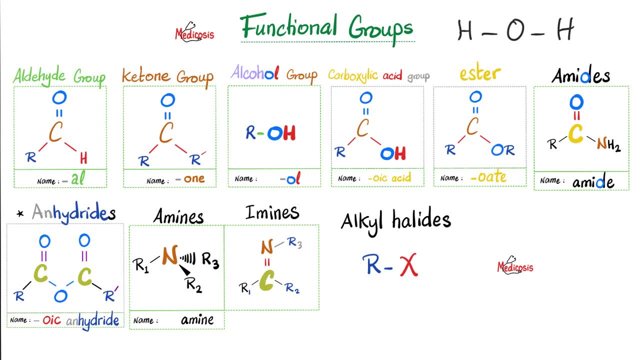 end in O Alcohols. end in O Carboxylic acids. end in Oic acid. Esters. end in O-8. Amides. end in amide Anhydrides: the name ends in Oic acid because anhydrides result from condensation. 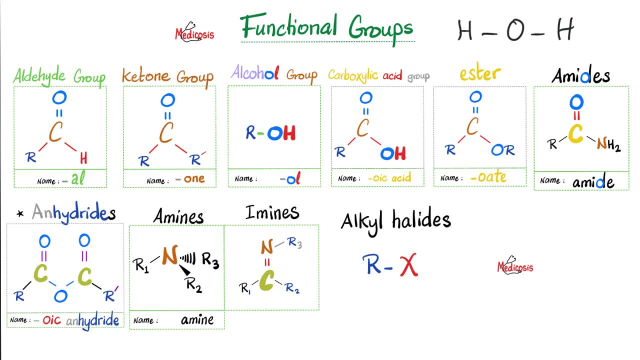 which is a combination of two carboxylic acids: Oic anhydride N means no, or removal. hydro means water, because when you condensate or you condense two carboxylic acids together, water is gonna leave the chat and this will be an anhydride- no water. 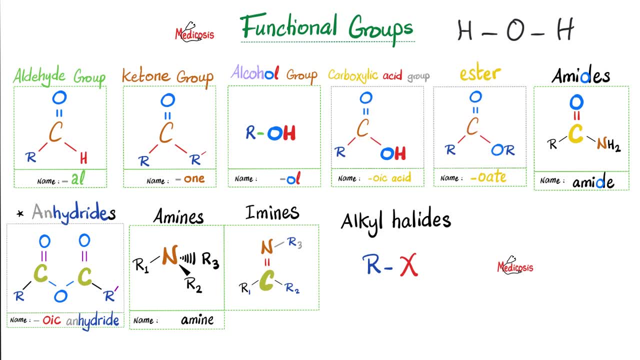 Esters, and instead of C-O-O-H it is C-O-O-R. I replace the O-H with O-R. That's why ester is a carboxylic acid derivative. I'm derived from almost the same formula. Look at this: O-H. 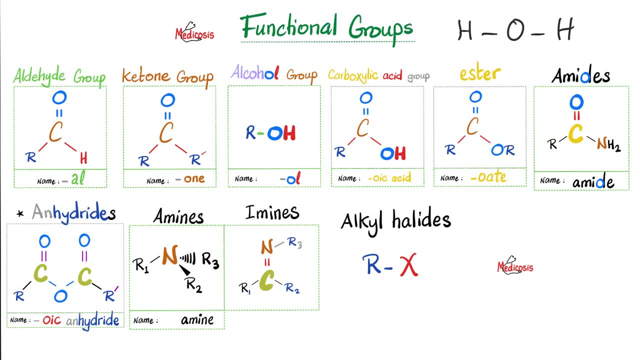 it plays with O-R. The rest is history. How about amides? Instead of O-H, put N-H-2.. Okie-dokie, So amides are also carboxylic acid derivatives. The word M or amy reminds me of amino So. 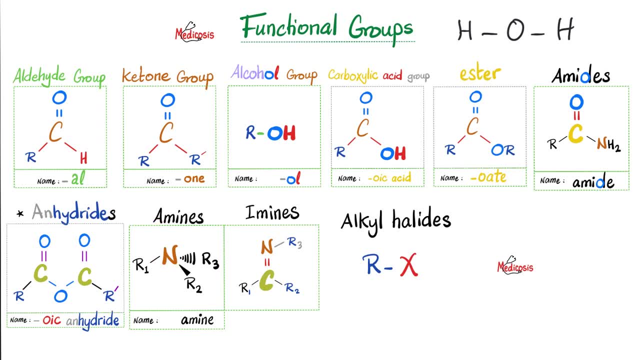 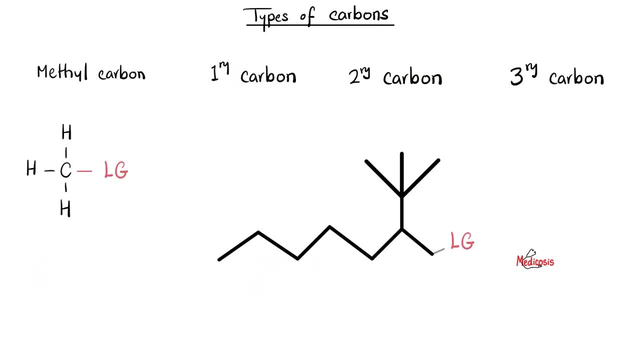 think of nitrogen. Look at this. A-M-I Think of nitrogen. Okay, let's tweak it a little. E-mine: Oh, it's nitrogen, but it's double bonded to carbon Carbon types. Look at this: Oh, CH3 is. 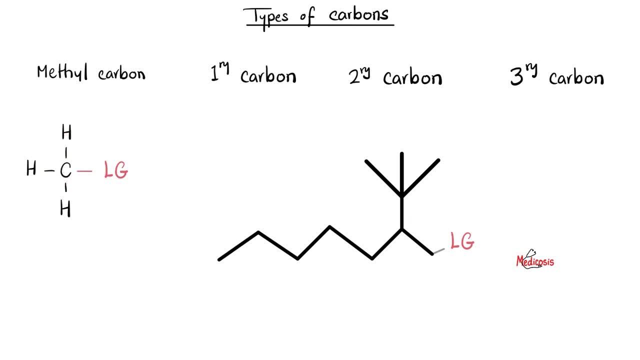 called methyl. All right, so this is just the methyl carbon, All right. How about primary carbon versus secondary carbon, versus tertiary carbon? Easy: If the carbon is communicating with only one other carbon, it's primary carbon. If the carbon communicates with two other carbons, it's a secondary carbon. If a carbon communicates: 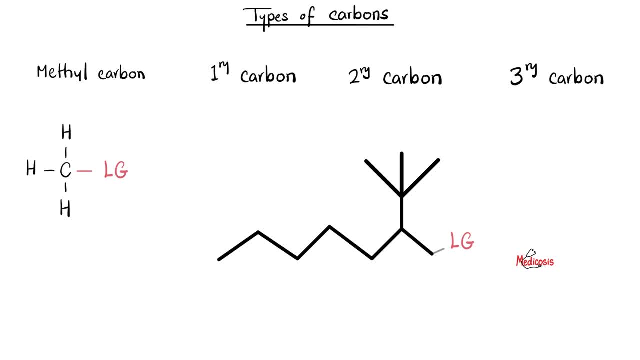 with three other carbons, it's a tertiary carbon. Let's practice. Look at this carbon right here. It's a carbon that communicates with only one carbon. So this carbon right here is primary carbon. How about you, this carbon? 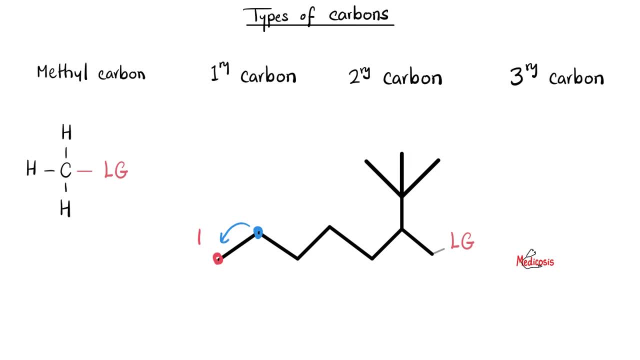 Well, I, As a carbon, I connect with this carbon on this side and this carbon on that side. I connect with two. I am a secondary carbon. How about this doozy carbon right here? Let's think about it, I'll give. 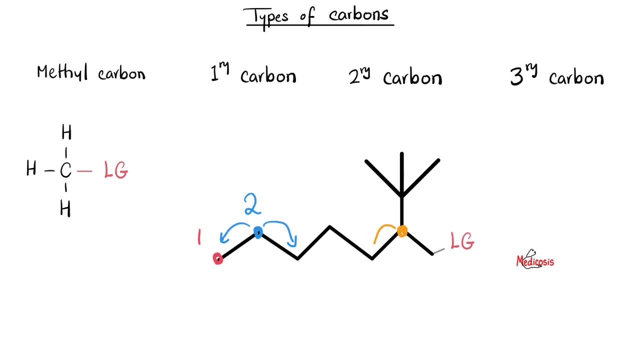 you a moment to think about that. Okay, I as a carbon, I connect to one carbon, second one and third one, So I am a tertiary carbon. As for this carbon right here, it communicates with one, two, three and four, So this is a quaternary carbon. 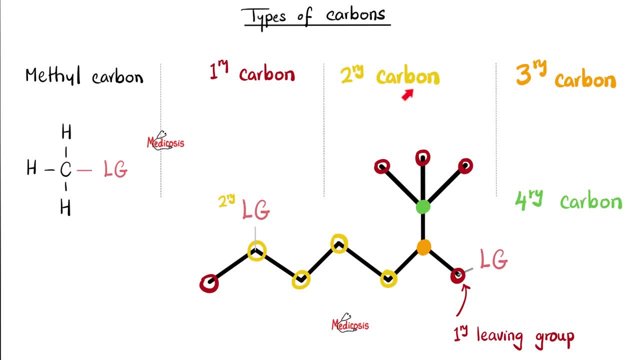 Primary carbons with this color, secondary carbons with the yellow color, tertiary carbon with the orange color and the quaternary carbon with the green color. Pause and review. How about this carbon? right here, It communicates only with one, so it's a primary carbon, And 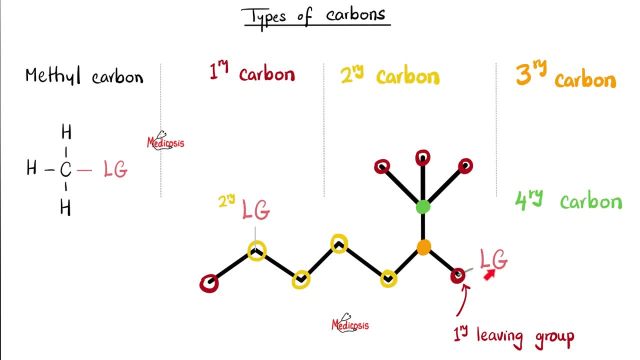 if you have a group that's bonded to a primary carbon, we call it primary leaving group. Let's say that we have a leaving group attached to the secondary carbon, then this will be called secondary leaving group. Forget the leaving group, Let's make this OH, which is 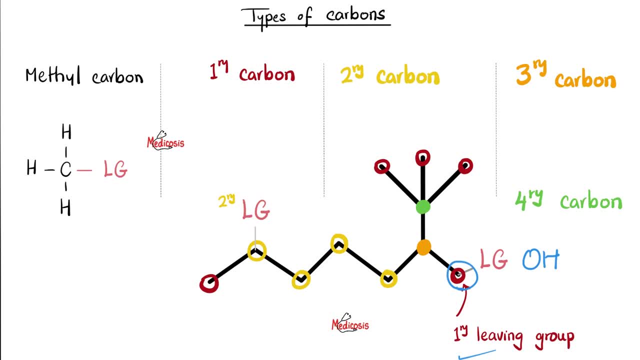 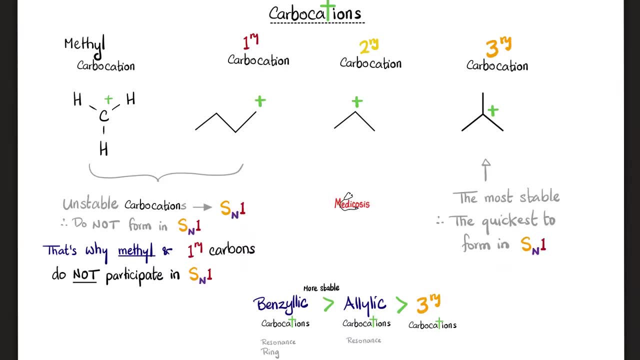 an alcohol group. If the OH is attached to a primary leaving group, this will be called primary alcohol. If the OH is attached to a secondary leaving group, it will be called secondary alcohol. The same story applies for the positive carbocation. This positive is on. 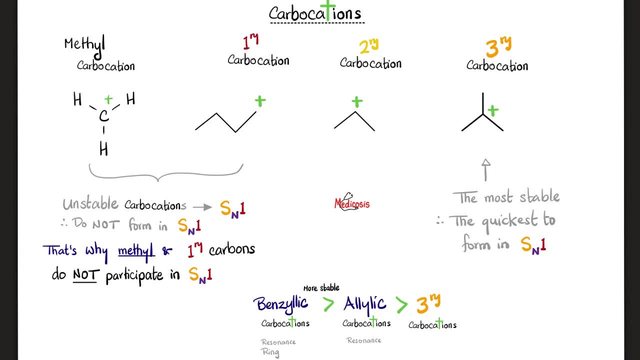 a primary carbon because this carbon is attached to only one other carbon, So it's called primary carbo carbon cation positive charge, This one. okay, look at this carbon. One carbon here, one carbon there. It's a secondary carbon. 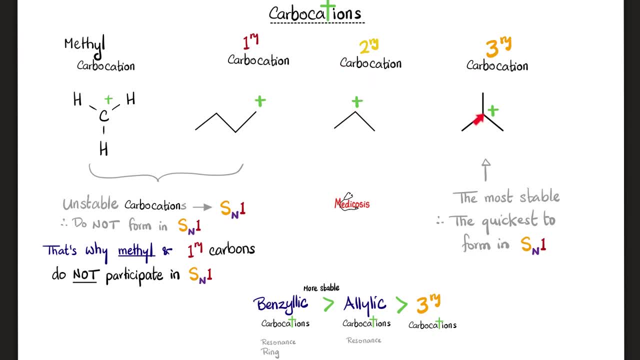 So this is a secondary carbocation. How about this One, two and three? It's a tertiary carbon, So this is a tertiary carbocation. Why is this positively charged? For this you need to calculate the formal charge. Let's just draw a carbon and let's draw the remaining. 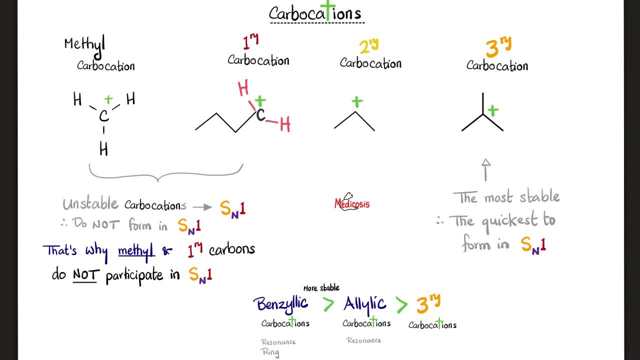 hydrogens. In this case, only two hydrogens remain. Okay, to get the formal charge. first you write down the number of bonds or the number of valence electrons that you expected to find in reality. Let's look at carbon. Carbon should make four bonds correct. Yes, 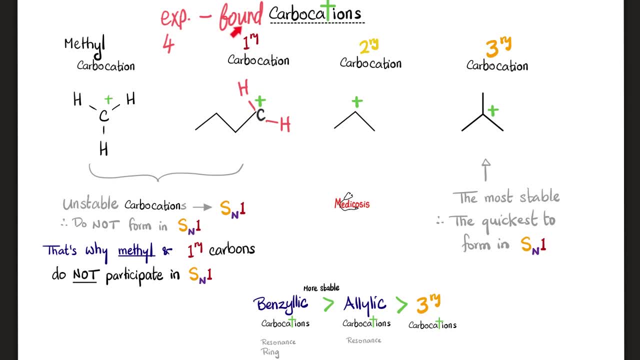 it should make four bonds. Let's look at what actually happened in reality. When I looked, I found one, two and three. I only found three. So four minus three equals positive one. Hence a positive one charge on this carbocation, And this is how to calculate the formal charge. 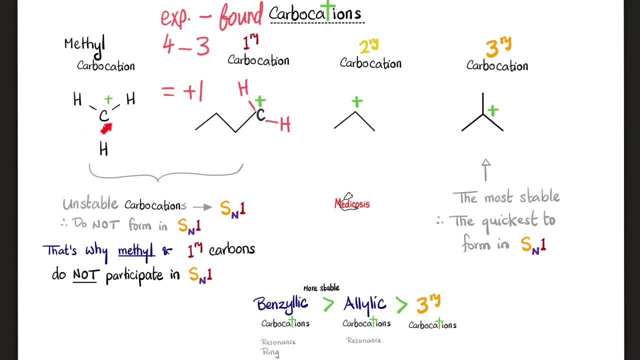 What you expected minus what you found. You can try it again here. Carbon should make four. This is what I expected. Look in reality, here it's one, two, only three bonds, Only three valence electrons. So four minus three is positive one, Positive one. 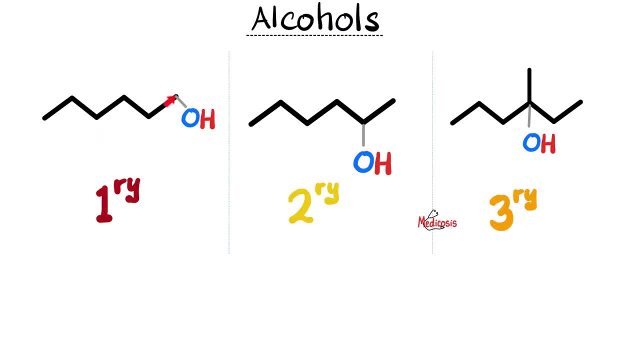 charge Carbocation. Look at this OH: It's on a primary carbon, So it's a primary alcohol. This OH, this hydroxy, is on a secondary carbon, So it's a secondary alcohol. And this is a tertiary alcohol because the OH belongs to a tertiary carbon, which is a carbon connected. 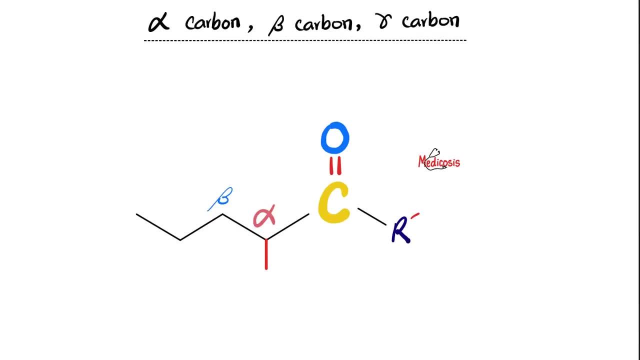 other carbons. Now, please do not confuse primary carbon, secondary carbon, tertiary carbon with alpha carbon, beta carbon and gamma carbon, because they are two different systems. You see this? This is called the carbonyl, which is carbon double bonded to oxygen. We saw this in the 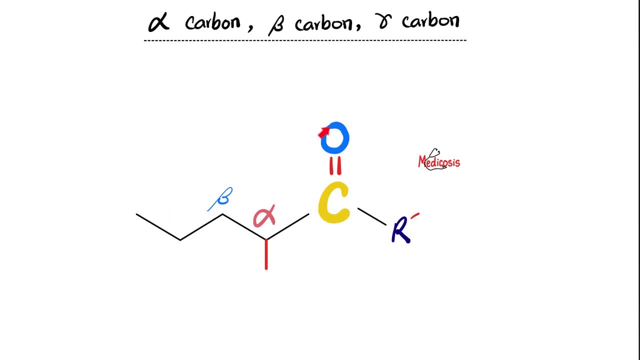 aldehydes, in ketones, in carboxylic acids and esters and amides and anhydrides. This carbon of the carbonyl is ground zero, okay. Next to it is carbon alpha, or the alpha carbon. 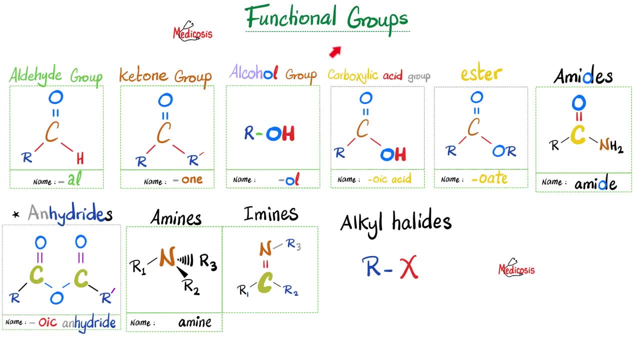 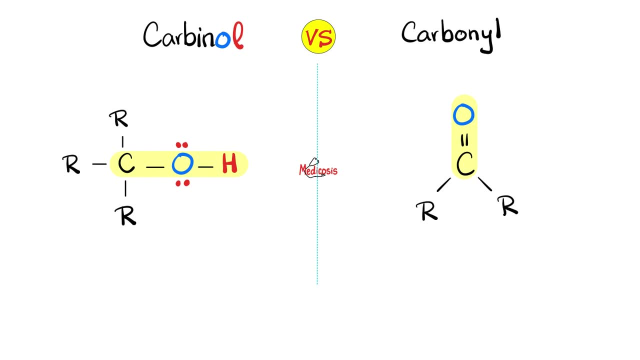 And then the beta carbon, the gamma carbon, etc. Here are the famous functional groups again. This is not a comprehensive list, but these are the most important ones for your exam. Another important distinction is carbonyl versus carbonyl. Carbonyl- it's an alcohol group. Here's: 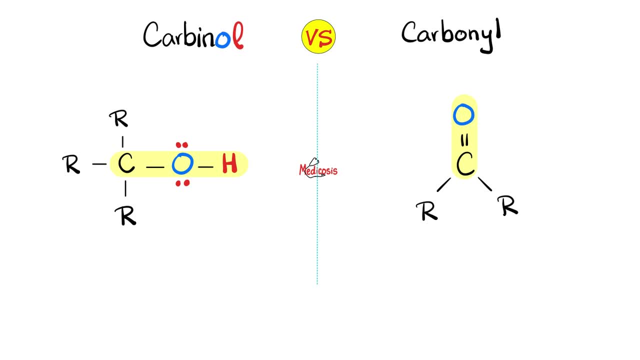 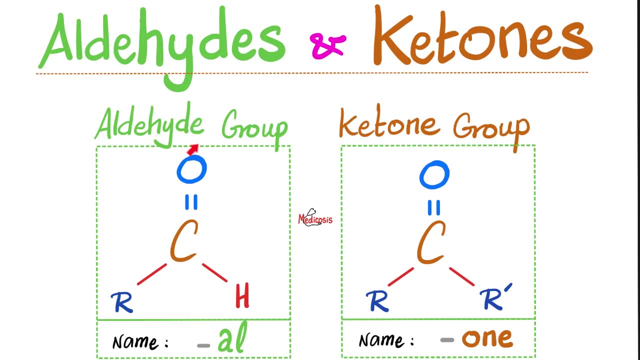 the R. rest of the chain, OH alcohol group. But carbonyl is carbon double bonded to oxygen, not carbon single bonded to OH. Aldehydes look like this COH, but ketones look like CO. And then instead of the H I have another chain, Aldehydes and an L. 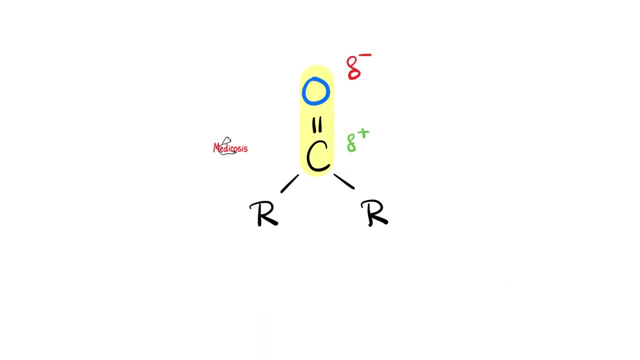 ketones and an ON. Here is the carbonyl which is found in aldehydes, ketones, carboxylic acids and the derivatives of the carboxylic acids, which are esters, amides, anhydrides. Since I have 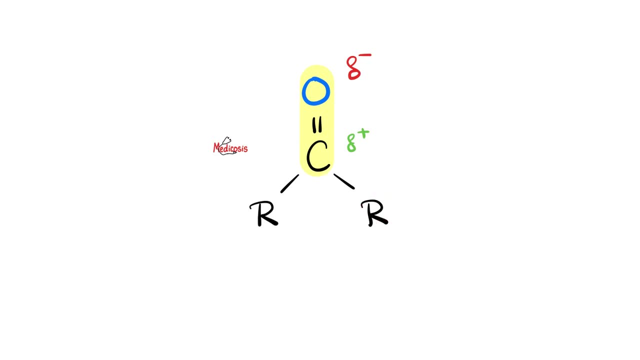 rest of the chain here alcohol chain. here this is a ketone. Do you remember the periodic table? Yes, I had carbon followed by nitrogen, then oxygen, then fluorine, And electronegativity increases this way, meaning oxygen is more electronegative. 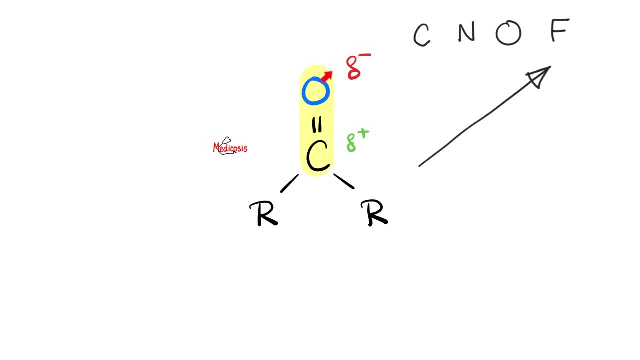 than carbon. Oxygen is more electronegative than carbon. Oxygen loves the negativity more than carbon, So the negative electrons will be attracted more towards the oxygen and away from the carbon. creating what? Creating a dipole. And we draw the arrow like this: The head of the arrow is: 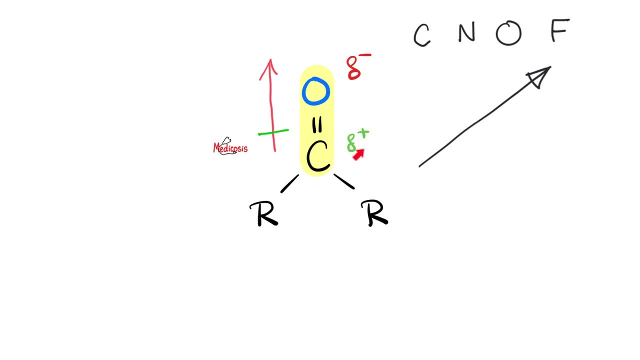 the negativity. And this plus sign is for the partially positive Oxygen and partially positive carbon. Now imagine that we have something negative, Let's say a nucleophile, which is negative. Nucleophile is negative. Of course the negative will be attracted. 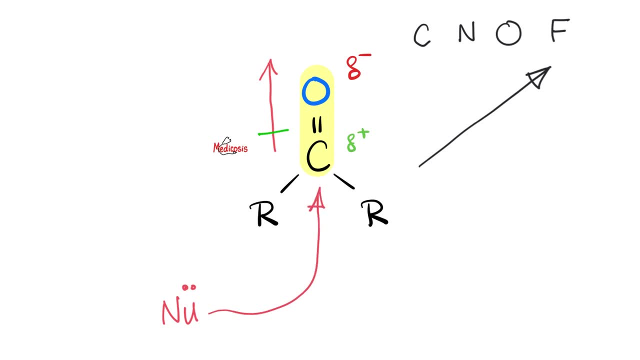 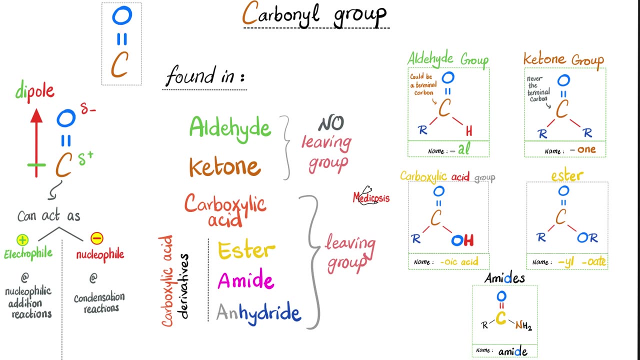 to the partially positive carbon of the carbonyl group. Again, what are the functional groups that contain this carbonyl, which is carbon double bonded to oxygen? You find this in aldehydes. You find this carbonyl in ketones. You find it in carboxylic acids and the derivatives of the. 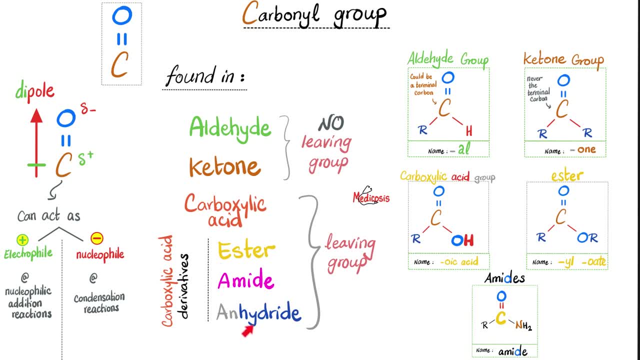 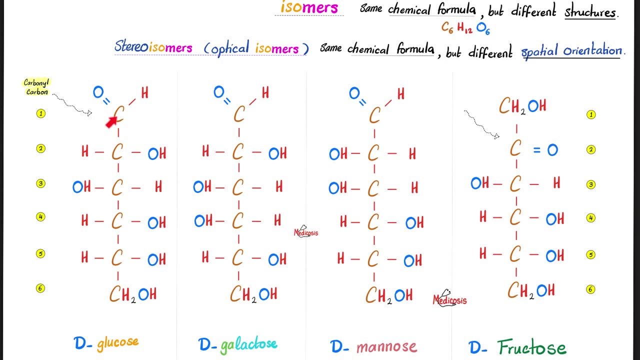 carboxylic acids, which are esters, amides, anhydrides. In this situation, the oxygen is becoming partially negative and the carbon is becoming partially positive due to electronegativity difference. You see this? D-glucose, Oh, C-H-O. Oh, this is an aldehyde. Yes, Aldehyde group could. 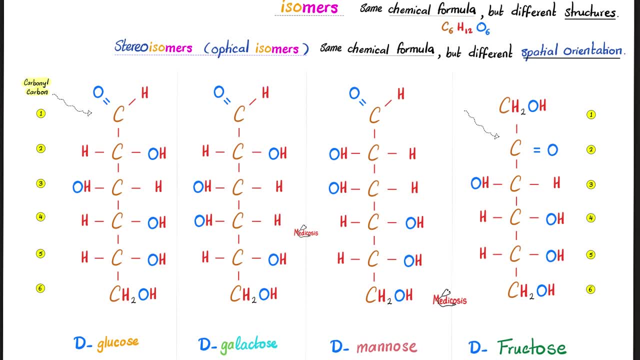 exist on carbon number one, the first carbon in the chain. However, look at D-fructose, which is a ketone. Oh, look at this carbonyl, That's a ketone. Here I have an alkyl group. here's an R and here's an R. Rest of the chain. rest of the chain. 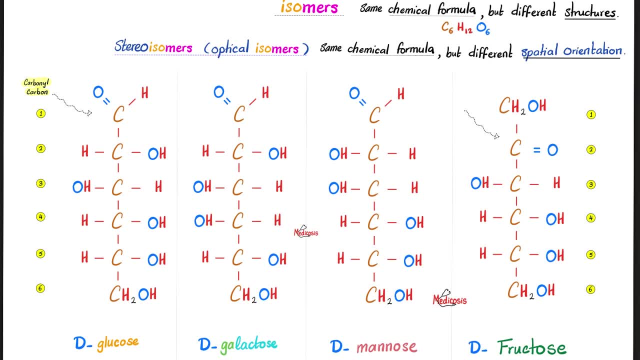 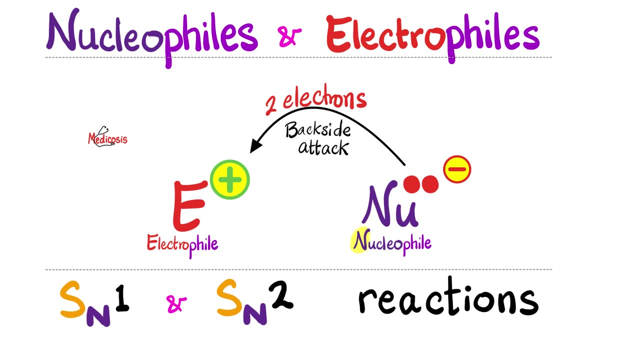 on both sides. that's a ketone. Ketone carbonyl can never be on the first carbon Carbon two, yeah, maybe Three, it can happen, but never on the first carbon. Next, nucleophiles versus electrophiles. Remember, nucleophiles are negative. 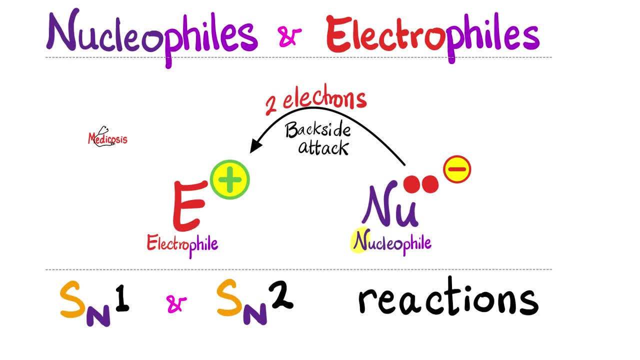 and electrophiles are positive. Why are nucleophiles negative? Because they have negative electrons, Excess pair of negative electrons. This pair will go from the negative to the positive because the negative is attracted to the positive. The arrow is always going from the nucleophile. 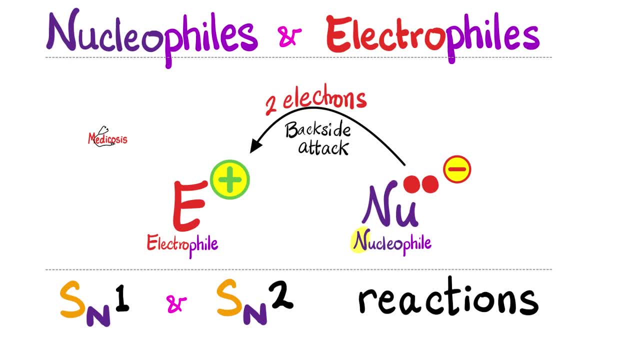 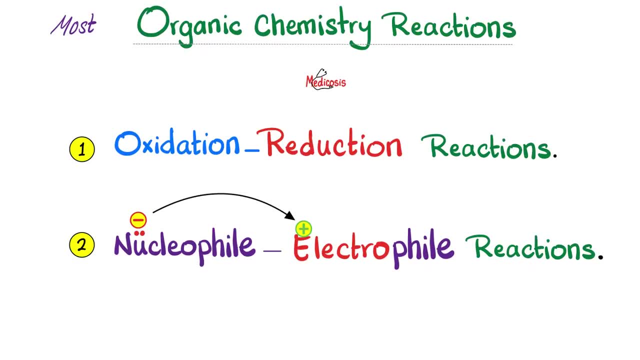 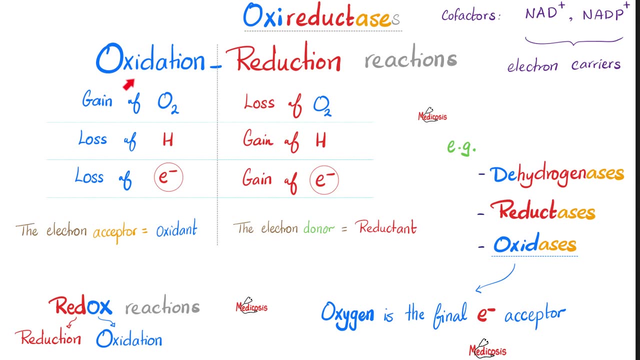 to the electrophile, which means the electrons are always going from the negative nucleophile to the positive electrophile. Organic chemistry reactions could be divided mainly into two categories: oxidation reduction reactions and nucleophile-electrophile reactions. Oxidation reduction: What is oxidation Oxidation in chemistry? 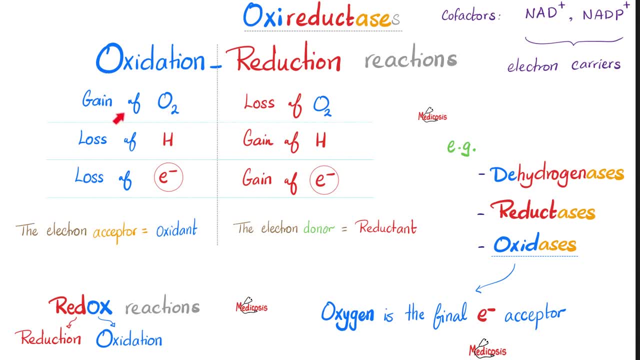 could mean one of three things: Gain of oxygen or gain of a bond to oxygen, loss of hydrogen or loss of negative electrons. Reduction is the opposite. loss of oxygen, Oh yeah, because when you gain oxygen you are oxidized. 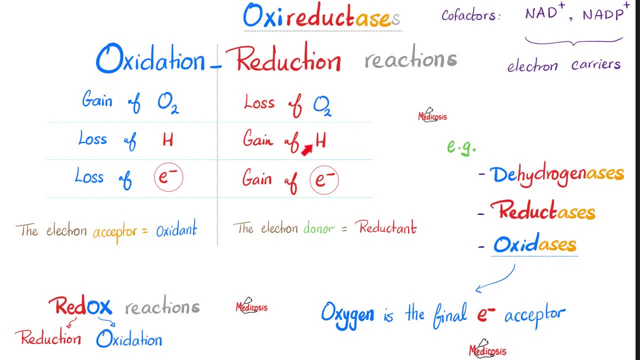 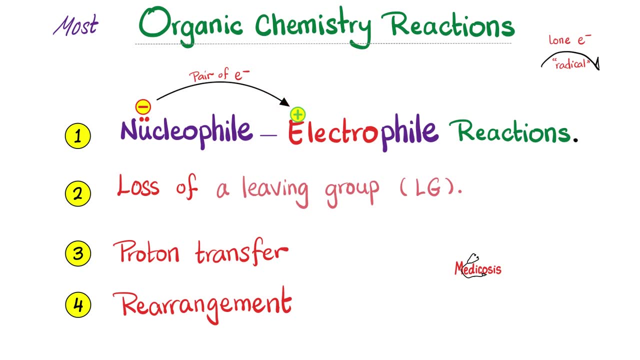 but when you lose it, you are reduced. It could be gain of hydrogen or gain of negative electrons. Next, nucleophiles versus electrophiles. Look at this arrow. it means what? It means that the electrons are moving from the nucleophile to the electrophile. 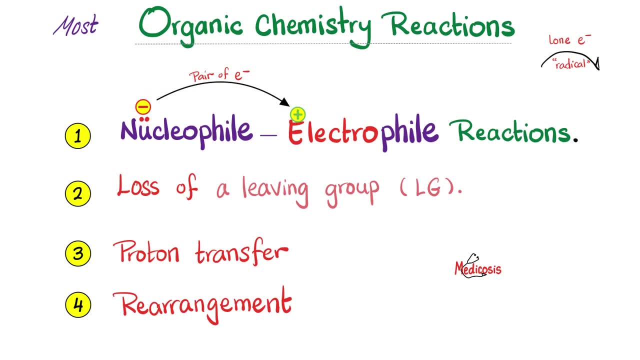 Electrons are moving from the tail of the arrow to the head of the arrow. When the arrow is complete, like this, it means two electrons or one pair of electrons is moving. But when it's half an arrow or a fish hook, like this, it means a lone electron. 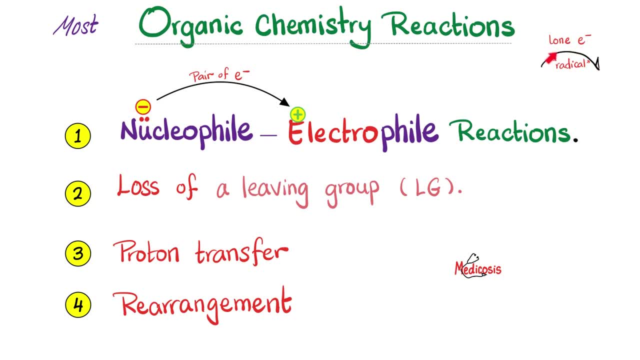 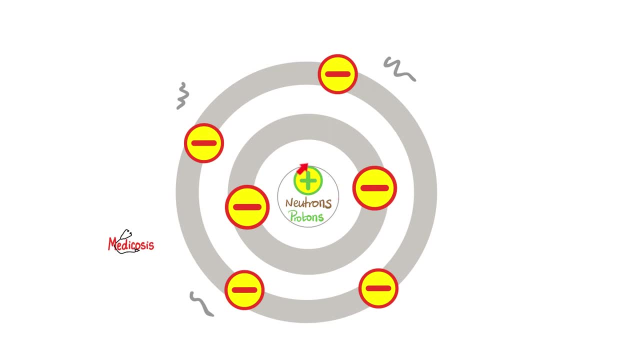 only one electron, not a pair, but one electron is moving. Why do we call them electrophiles and why do we call them nucleophiles? First let's go back to general chemistry. Remember that the nucleus is positive and the electrons around it are negative. 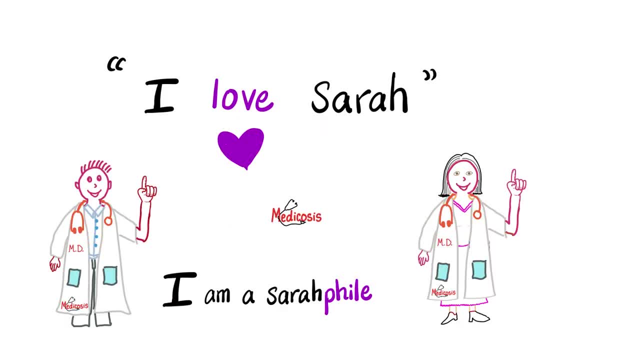 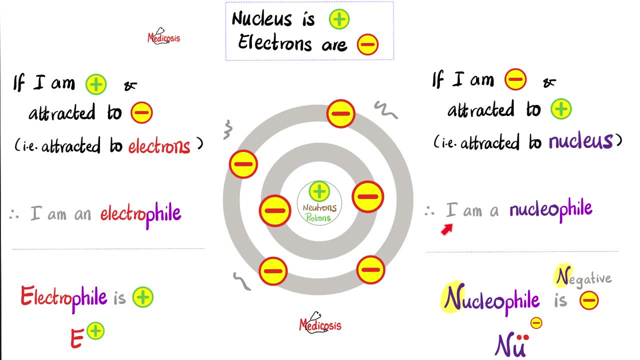 If I say I love Sarah, it means that I am Sarahphile, a lover of Sarah. So let's say that I am negative. If I am negative, I'll be attracted to the positive nucleus. I am a nucleus lover seeking the positive nucleus. If you seek the positive nucleus, 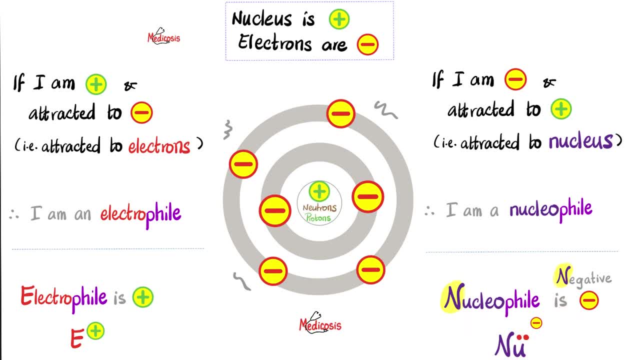 you're a nucleus lover. nucleophile You're negative, but you love the positive nucleus. That's why they're called nucleophile. Conversely, if you're electrophile, it means that you are positive but attracted to the negative electrons. When you're attracted to the negative electrons, you're electrophilic. 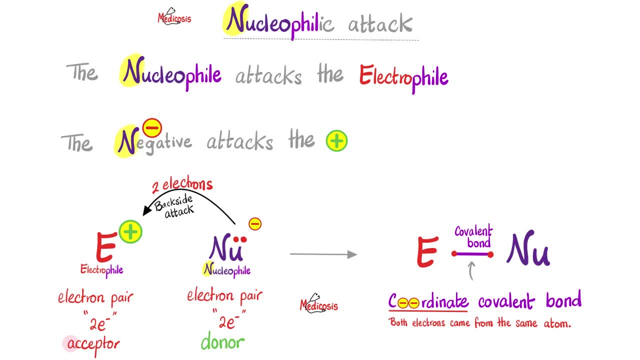 Mnemonic, to keep it easy. Nucleophiles are negatives. Conversely, electrophiles are positive. The negativity is here because the electrons are at the nucleophile. Then the electrons will move from the nucleophile by being attracted to the electrophile. 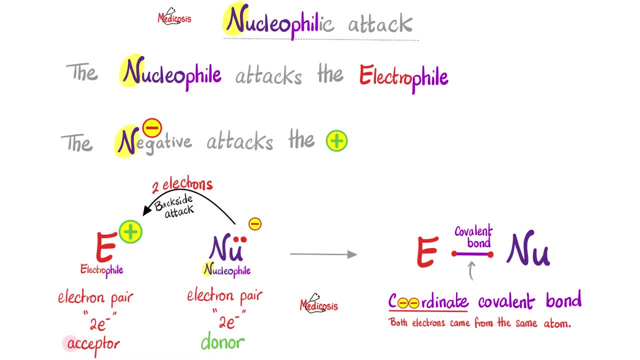 This is called a backside attack. When you see a complete arrow like this, it means that the pair of the electrons are moving. What's the result? The result is that I'll use this pair of electrons, which is two electrons in total, to make a new single covalent bond between the electrophile and the nucleophile. 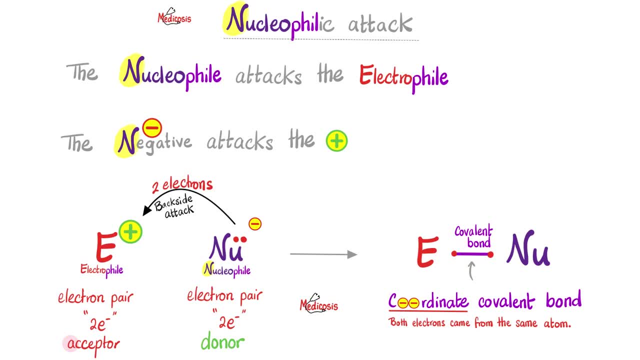 This is called coordinate covalent bond. I understand that it's a covalent bond, but why coordinate? Because both of these electrons that are making the bond here came from one group. In this case, it came solely from the nucleophile. This pair of electrons did not. 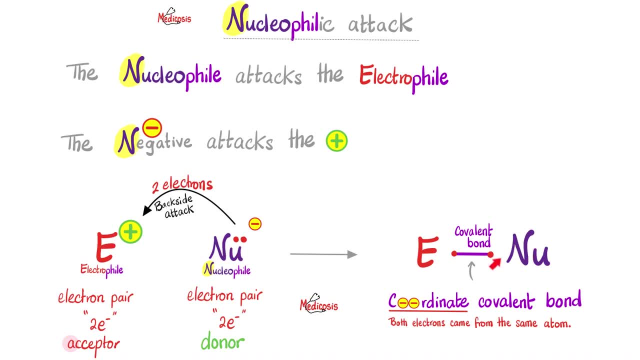 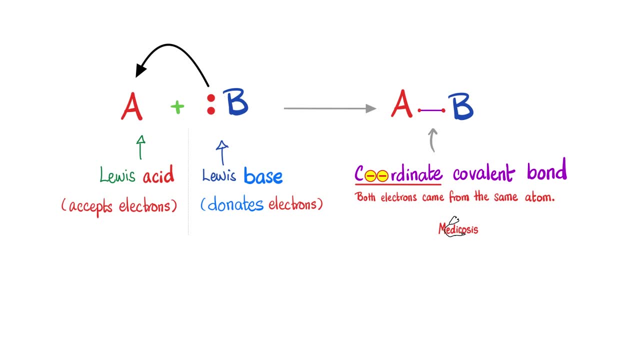 come from the electrophile at all. Both came from the nucleophile coordinate. Here is lovely atom. Here's another atom. Who has the electrons B, Who has the negativity Also B. So B will attack A Always. the nucleophile is attacking the electrophile. 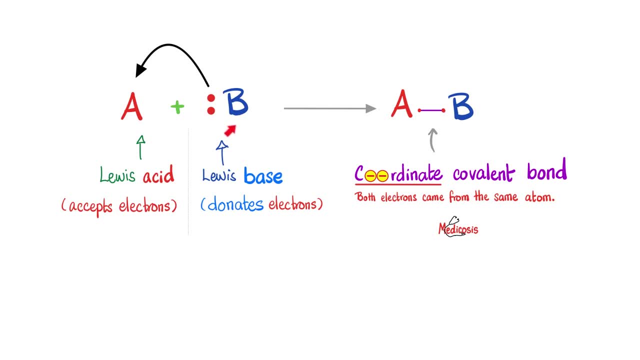 Nucleophile is negative. Why is this negative? Because it has an extra pair of electrons. Why is this positive? It does not have an extra pair of electrons, So the negative attacks the positive. Nucleophilic attack means the nucleophile attacks the electrophile. 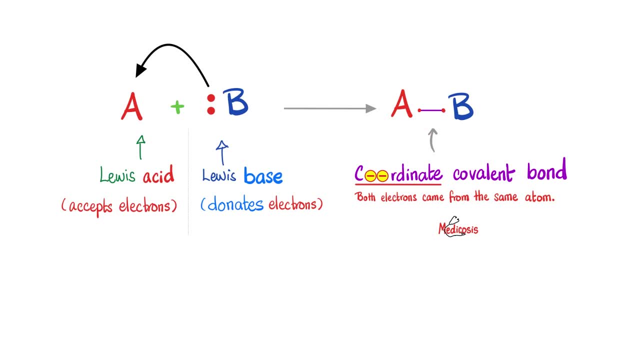 And then what? Use those two electrons to make a new covalent bond between A and B, between the electrophile and the nucleophile. Keep this idea in mind because we're coming back to this part: Acids versus bases- If you have watched my general chemistry playlist, 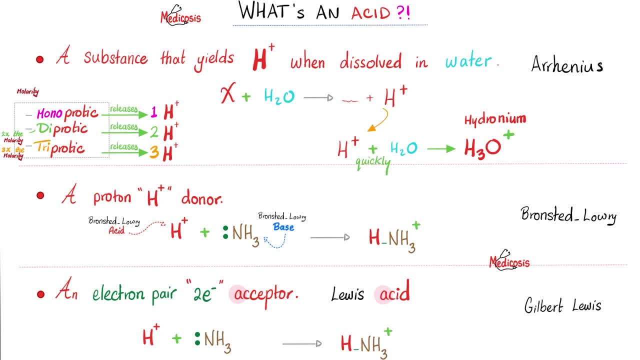 we have said that we have three definitions of acids. The Arrhenius definition, an acid is a substance that yields protons. Another definition, Bronsted-Lowry, is the acid is a proton donor. The Lewis definition is that the acid is an acceptor of electrons. The Lewis acid is an 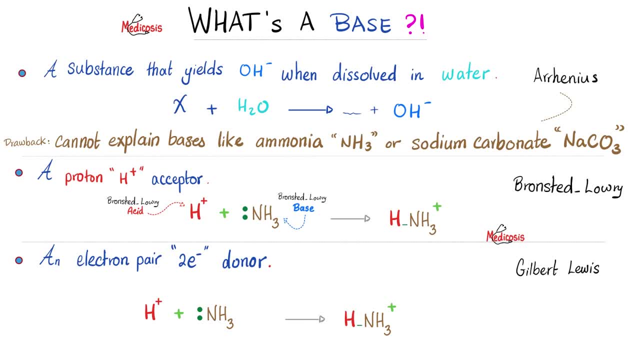 acceptor of electrons. Conversely, the base is the exact opposite. It yields the negative OH when dissolved in water. It's a proton acceptor, not donor. And the base is an electron pair donor, not an electron pair acceptor. It's an acceptor of electrons, but the Lewis base is donor of electrons. 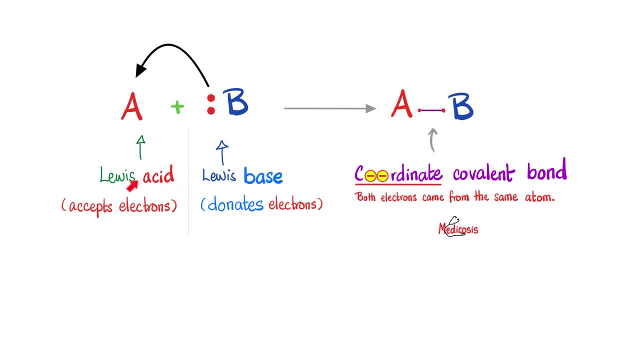 And we're back to the same slide. We just said that the Lewis acid is an acceptor of electrons and the Lewis base is a donor of electrons. Amazing, So this is the donor of electrons. It has an extra pair to donate. This is the donor of electrons. This is the Lewis base. 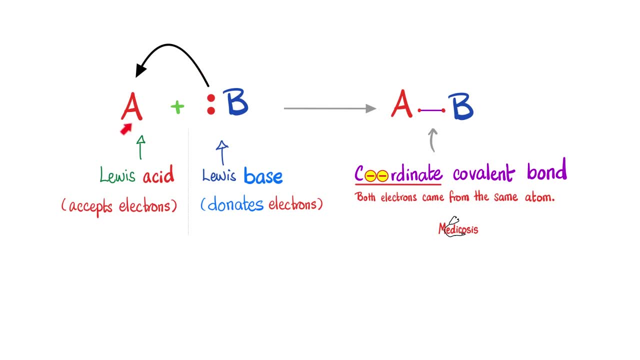 How about the A? The A will accept the electrons. It's a Lewis acid because it accepts electrons. So this is the Lewis acid and this is the Lewis base. But also, this is the electrophile and this is the nucleophile. Oh, therefore, a good nucleophile is usually a good base. 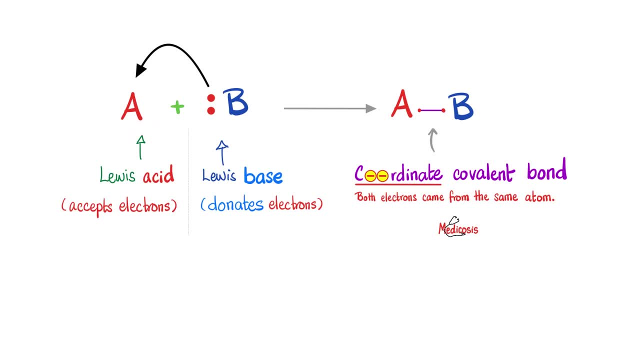 and the electrophile is usually an acid. How do I remember this? It's a meticulous mnemonic. You just write down the word Biden and let me tell you what this means. It's an acronym. The base, according to Lewis, is a. 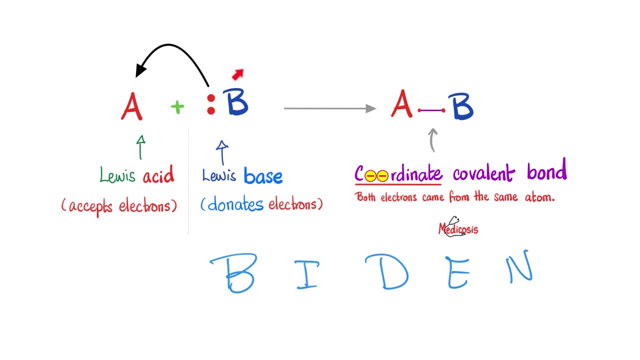 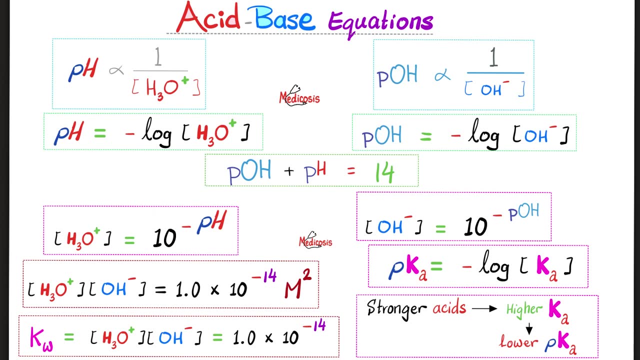 donor of electrons and it's also a nucleophile Negative. These acid-base equations are crucial. You need to know them by heart before you start organic chemistry. I've talked about them in detail in my general chemistry playlist. Don't forget that if I have a strong acid, it will have higher Ka but lower pKa. Why is this? 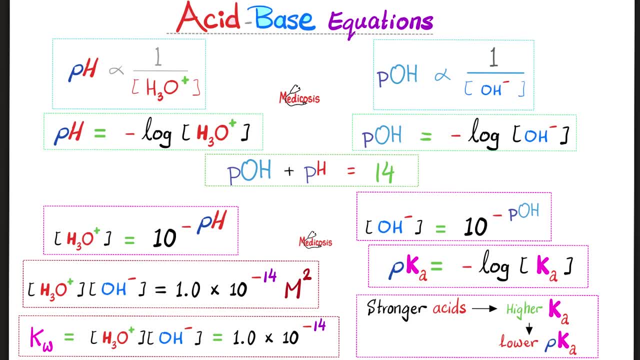 Because the pKa is the negative log of Ka. Moreover, a stronger acid will have a high hydrogen ion concentration or high hydronium concentration. However, the stronger acid will have a lower pH, because the pH is the negative log of hydronium ion concentration. Strong acids have higher Ka, lower pKa. Stronger acids have 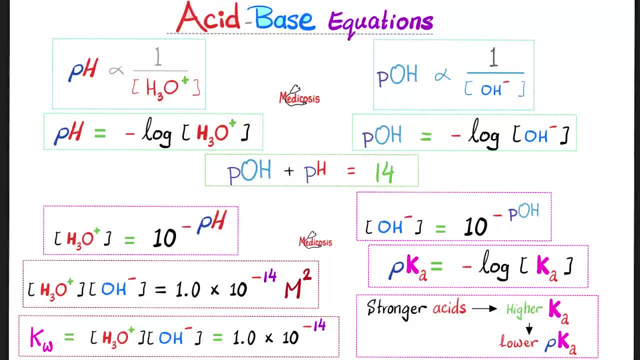 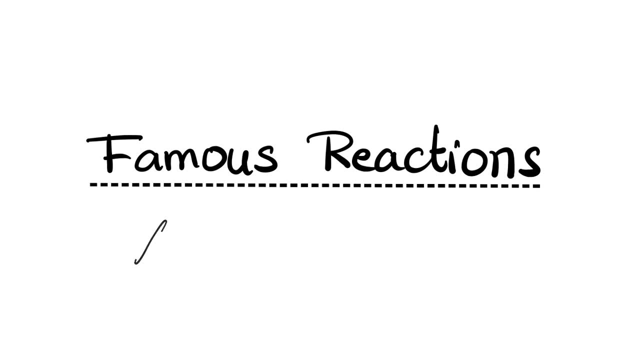 higher hydronium ion concentration but lower pH- Some famous reactions that you cannot afford to miss on your exam. On many exams, including the test, they give you molecule X reacting with molecule Y and they expect you to predict the product of this reaction. So here are some doozy tips. 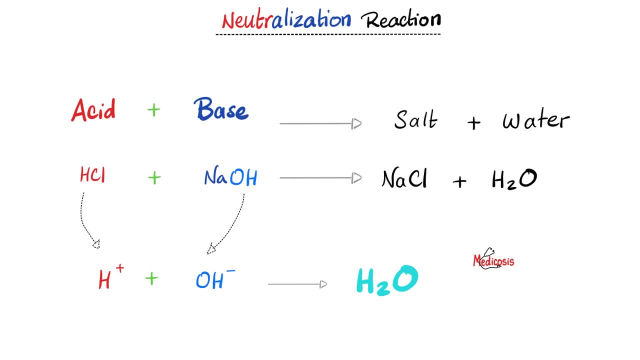 From general chemistry you know that acid plus base equals salt plus water. Never, ever forget this. Carboxylic acid plus base will give you the salt of the carboxylic acid plus water. Suppose that pentanoic acid reacted with a base, NaOH. what do you get? Well, it's. 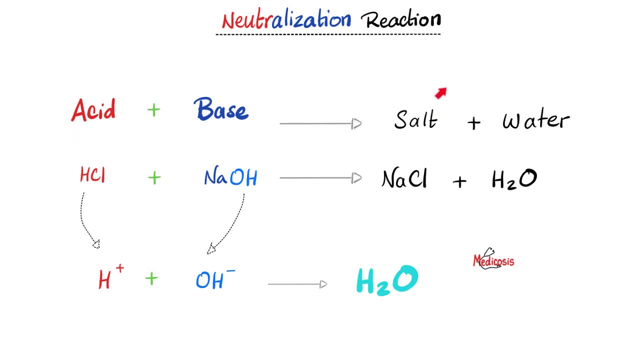 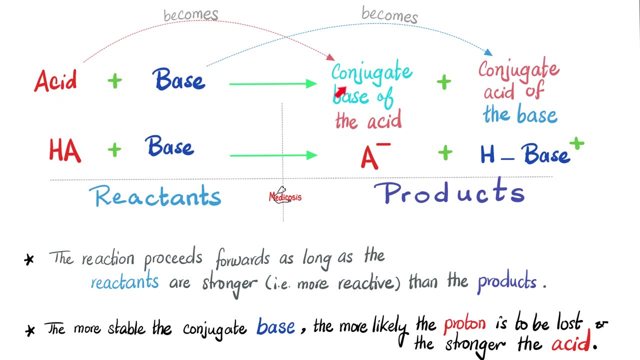 called pentanoic acid, I'll get NaOH plus water Also. acid plus base will give me the conjugate base of the acid and the conjugate acid of the base, Which means the acid, as it loses the protons, becometh the conjugate base of the acid And the base as it acquires the proton. 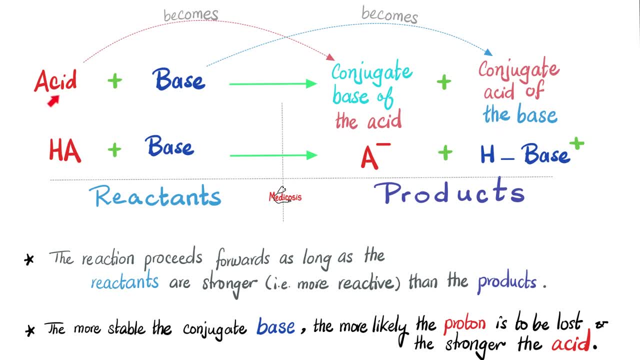 becometh the conjugate acid of the base. As the acid loses its protons, it becomes a negative, Because the proton that you lost was positive. When you lose the positive, you become a negative conjugated base. Conversely, as the base acquires that proton, 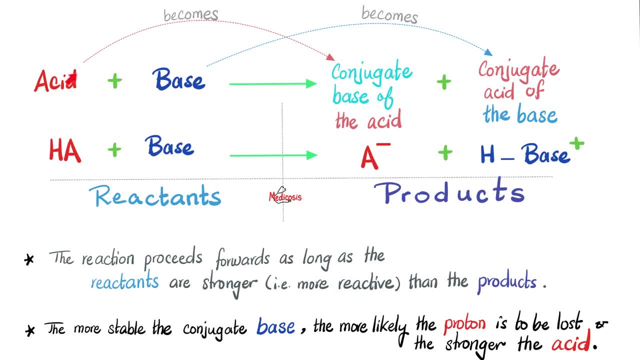 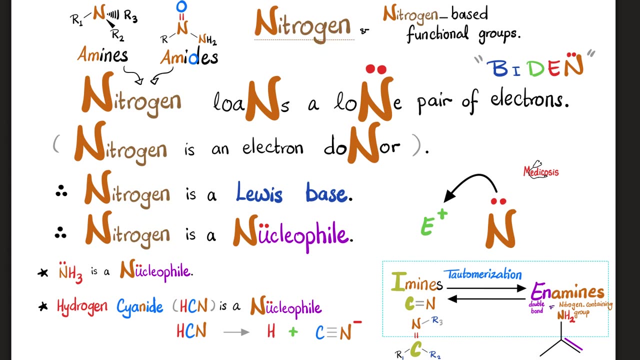 it becomes positive Because proton is positive. The acid will accept electrons, but the base is an electron donor. When you lose the electrons, when you lose the negativity, you become positive. An important mnemonic to remember forever is that nitrogen is nucleophilic. Why? Because nitrogen has 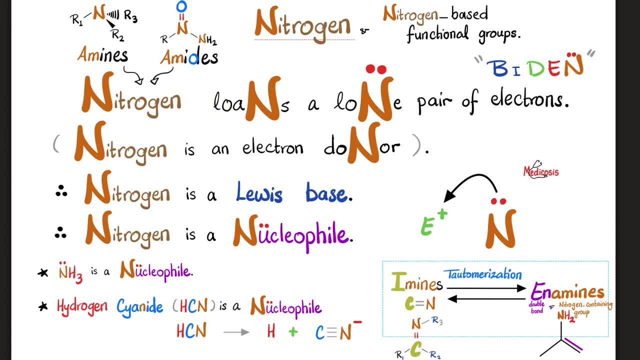 a lone pair of electrons that it can loan and give to others. And when you have a lone pair of electrons that you can give to others, you are a nucleophile by definition, And good nucleophiles are good bases, Strong bases, It's the same mnemonic Biden, again The base, according to: 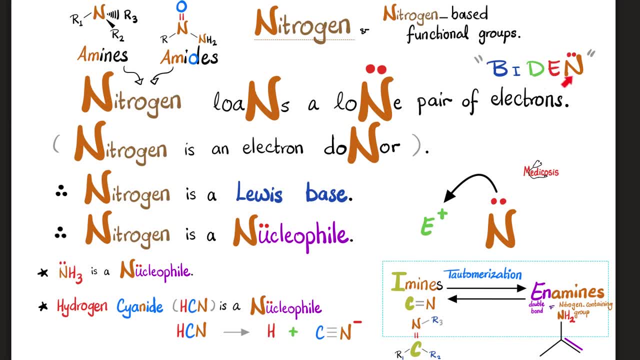 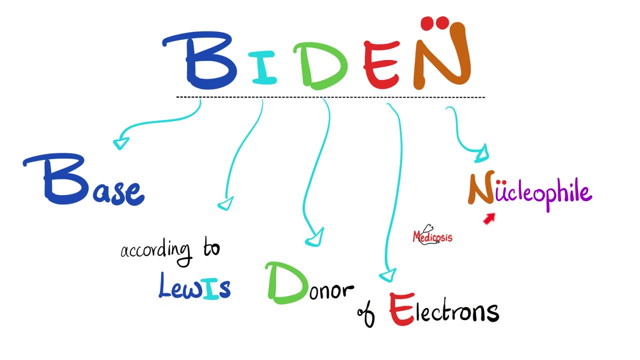 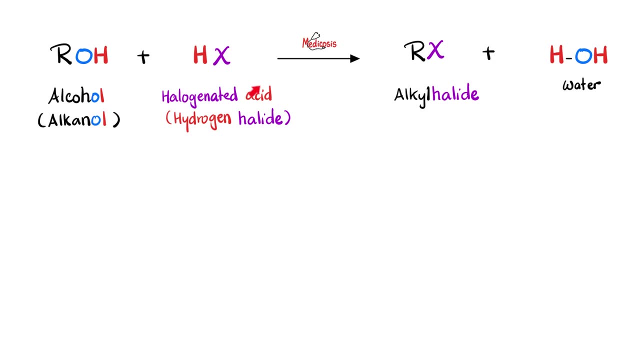 Lewis is a donor of electrons and is a nucleophile, which is negative. Base, according to Lewis, is a donor of electrons and is nucleophile, which is negative. Important reactions for your exam: When they give you an alcohol and a halogenated acid. 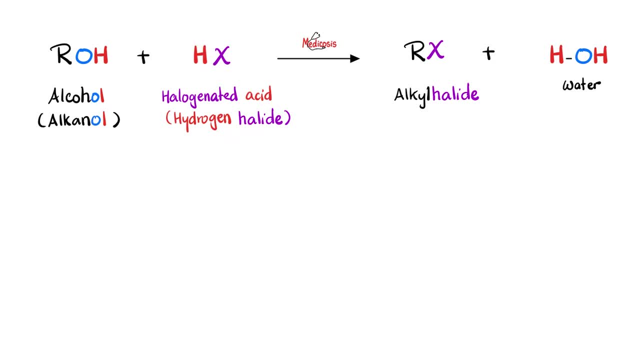 or hydrogen halide. a halide is a halogen, by the way, which means group 17 in your periodic table stuff like fluorine, chlorine, bromine, iodine, etc. It's a double substitution reaction. The R will take the X, lump them together and the H will take the OH and form water. 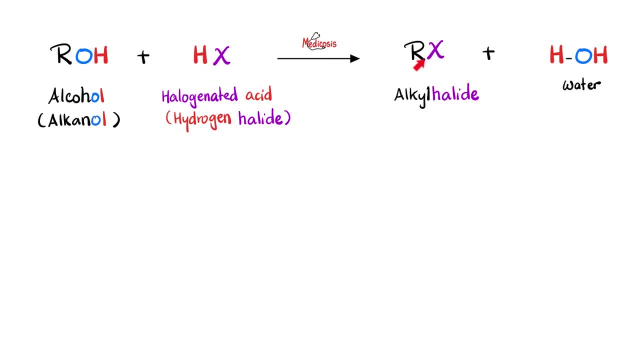 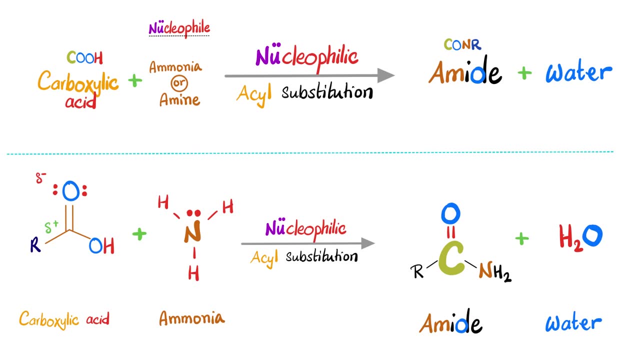 Alcohol plus hydrogen halide will give me alkyl halide plus water. Another gift for your exam that you cannot miss. When they give you carboxylic acid plus ammonia, you get amide plus water. I mean, think about it. If I have carboxylic acid which is COOH, 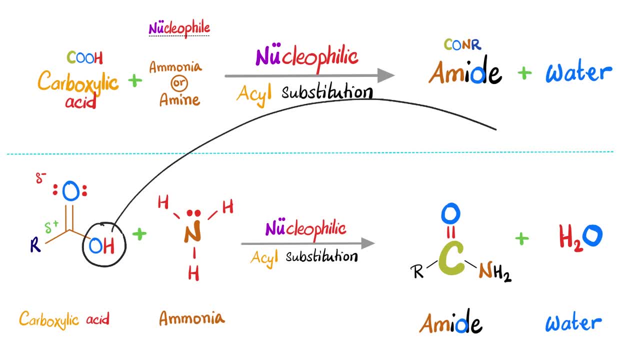 COOH. This OH is a leaving group. It will leave the chat to become part of water And in place of the OH, we'll put what We'll put NH2.. Amazing. What's that called? C-O-N-H-2 is an amide, not an amine. 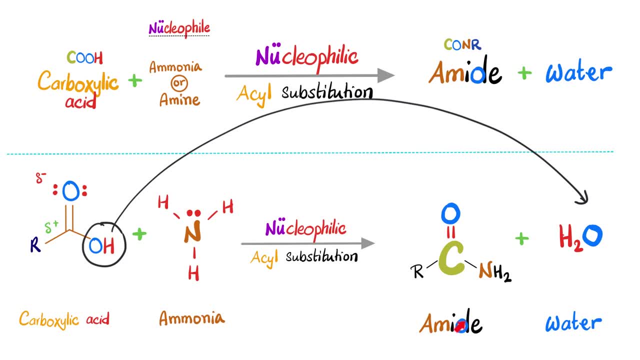 Because amide has a D, which has part of it that looks like an O, That's how I remembered- And M means what It's like: an amino. It has a nitrogen group. But hey, Miracosis, ammonia is NH3, but this is just NH2.. Yeah, because I took one H and help made the water. 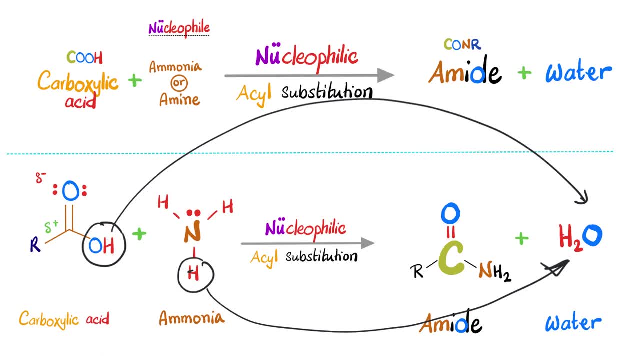 H from here, OH from there. Together you get H2O. What's that called Nucleophilic acyl substitution? Why substitution? Because the nucleophile substituted for the leaves. Why substitution? Because the nucleophile substituted for the leaves. 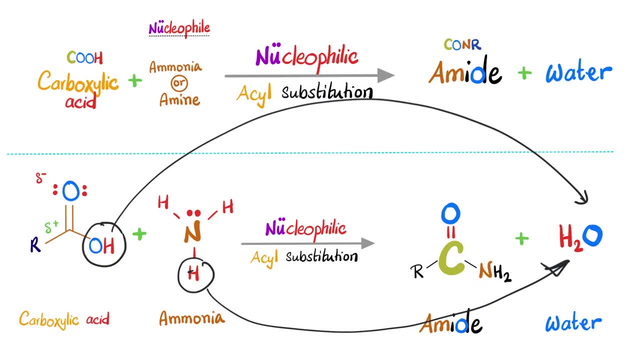 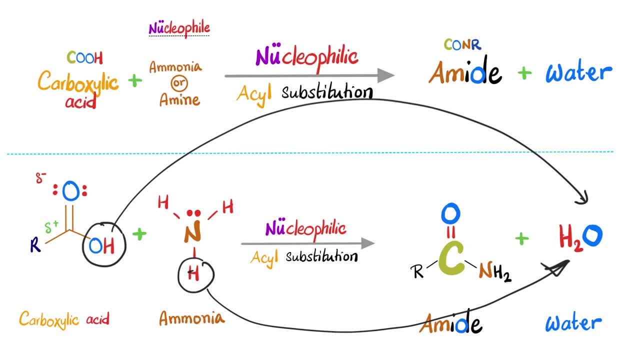 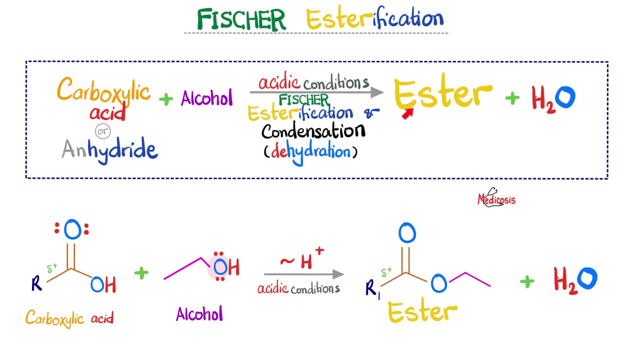 What are the derivatives of the carboxylic acids, Esters, amides, anhydrides? Another reaction that you should never miss is the fissure esterification: Esterification making ester From carboxylic acid and alcohol. Carboxylic acid plus an alcohol equals ester plus. 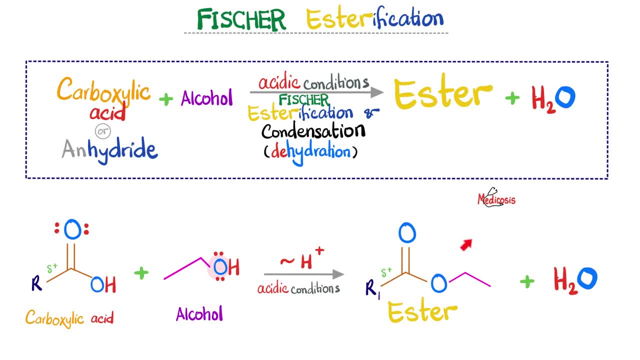 water. Here's a carboxylic acid. Here's an alcohol. Before you know it, I have an ester which is C-O-O-N-H-2.. Before you know it, I have an ester which is C-O-R plus water. 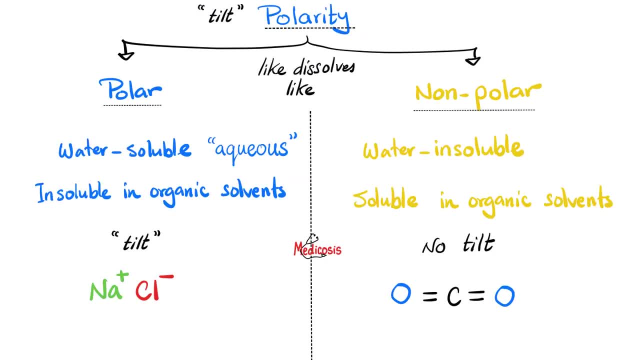 And this happens under acidic conditions. Polarity- What is polarity? Well, like dissolves. like: If you are like water, you'll be soluble in water. If you're polar, you'll be soluble in polar solvents, But you'll be insoluble in non-polar organic solvents. 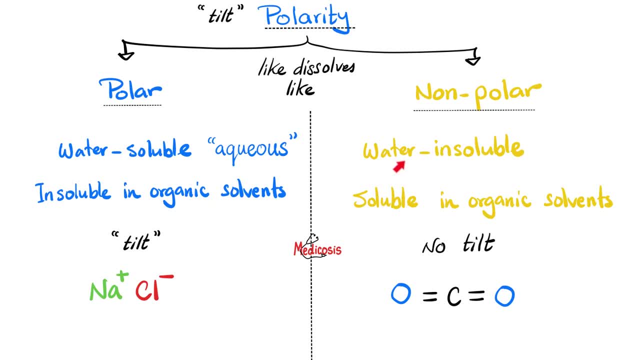 like benzene. How about non-polar molecules? They are water-insoluble, but they are soluble in non-polar organic solvents such as benzene. When they give you a molecule on your exam and they want you to predict whether it's polar or not, use my trick called the tilt. if you see a tilt, 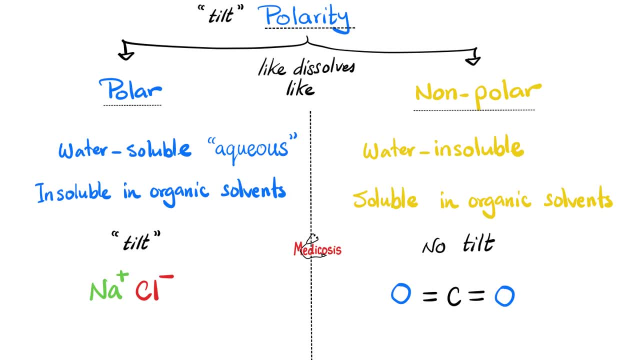 it's polar. if you see no tilt, it means non-polar. look at sodium chloride, for instance. i want you to cut it with a knife, just like this. do you see any difference between the left half and the right half? of course, one is positive, one is negative. that's a tilt, that is polar. but then look at this. 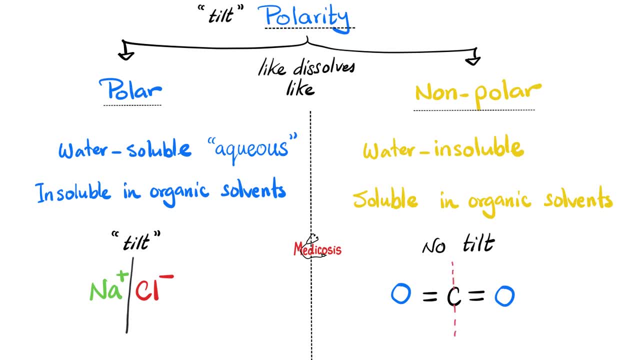 carbon dioxide. cut it with a knife, just like this. is there any difference between the left half and the right half? no, they are identical. there is no tilt whatsoever. no tilt means non-polar. this is polar and will be soluble in polar solvents like water. this is non-polar and will be soluble in. 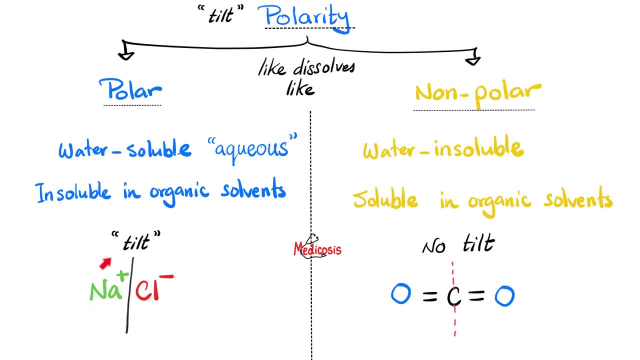 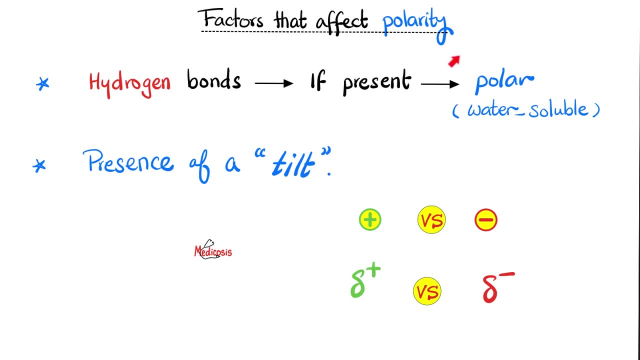 non-polar solvents like benzene. this will not be soluble in benzene and this will not be soluble in water. and, by the way, if you make hydrogen bonds, you're more likely to be polar and water soluble. if you have a tilt, you are polar. look at this. 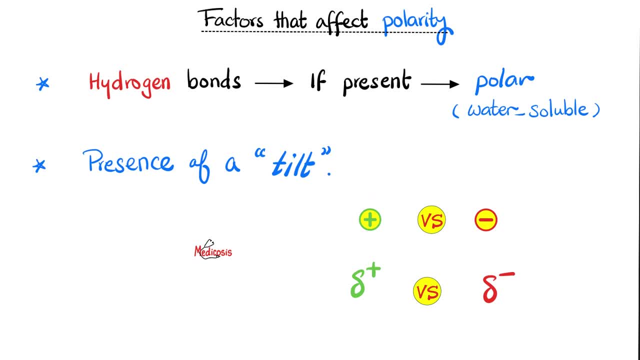 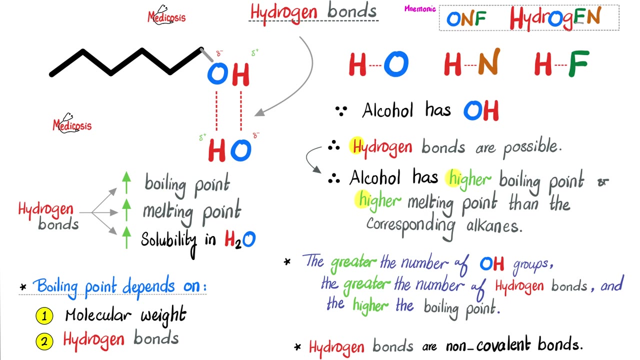 what's the tilt? it could be positive versus negative, like sodium chloride, or even partially positive and partially negative. polar, ionic, polar covalent. we talked more about this in my general chemistry playlist. hydrogen bonds can form between hydrogen and one of three molecules could be between hydrogen and oxygen, hydrogen and nitrogen or hydrogen and fluorine. how do i remember it? 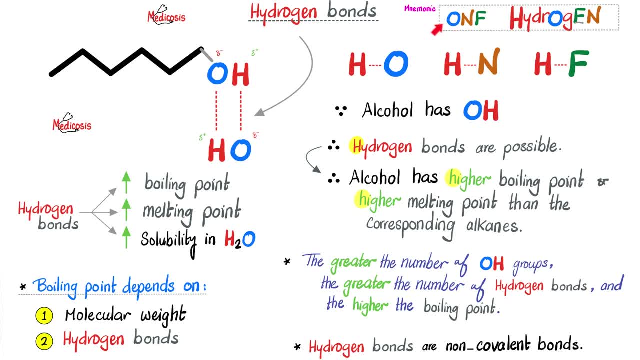 it's o and f or the oomph mnemonic hydrogen bonds. oomph oxygen, nitrogen or fluorine. another mnemonic is to write the word hydrogen funny. instead of a, just write it as if it resembles an f. and now hydrogen can make a bond with oxygen, just like this nitrogen, just like this or fluorine. 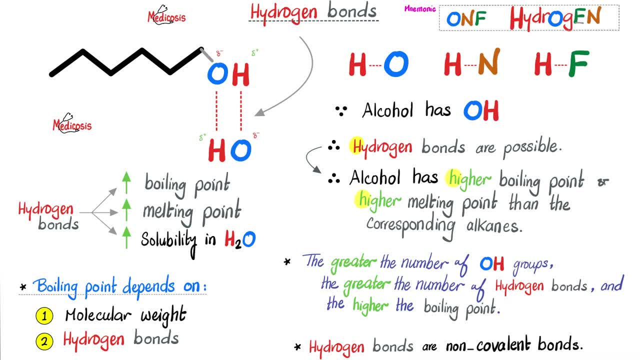 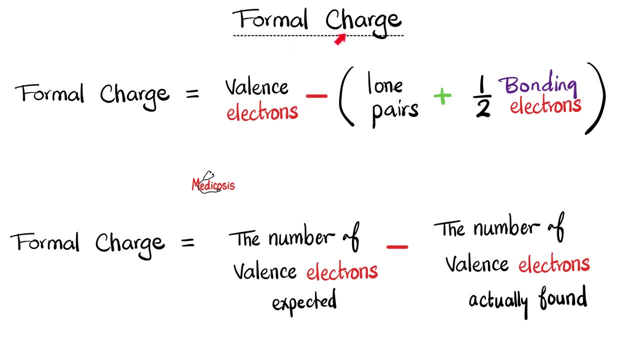 just like that, if you can make hydrogen bonds like alcohols, like carboxylic acids, you will have relatively high boiling point, melting point and high solubility in water, ie polar. now on the topic of formal charge again. now here's the technical way to do and calculate the 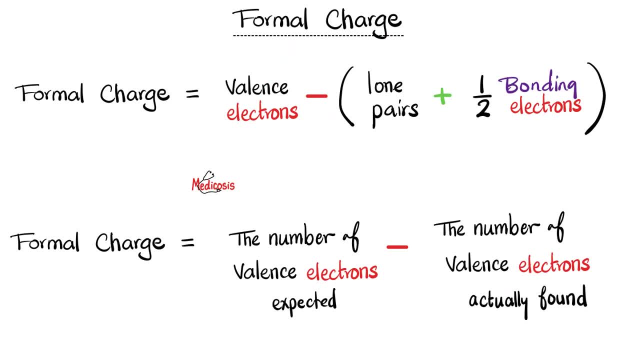 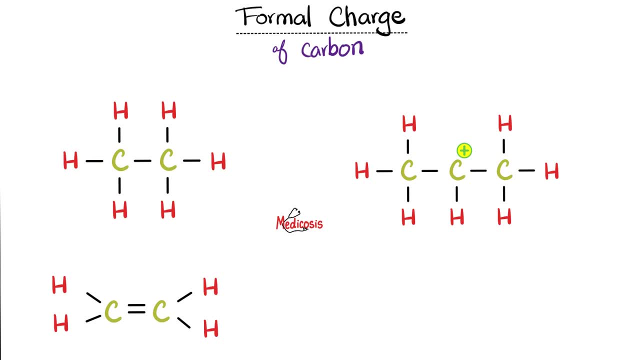 formal charge. you should ignore this and use the simpler version: what i expected minus what i actually found in reality. let's practice carbon. how many bonds do we have around carbon? what do we expect? we expect to have four. why is this? because hydrogen has six electrons in total. 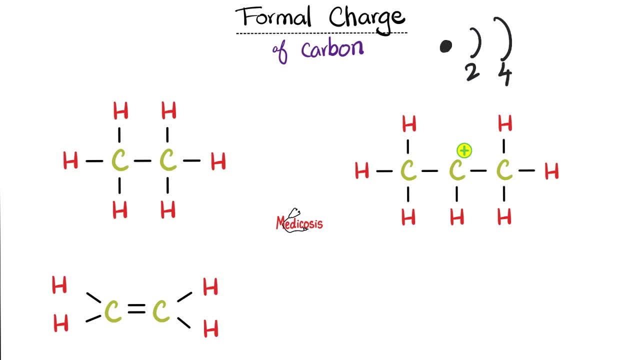 two will be in the first shell and four will be in the valence shell, so i expect four valence electrons, which means i expect four bonds. this is what i expected, minus what i actually found. one, two, three, four, four minus four is zero. this carbon atom is. 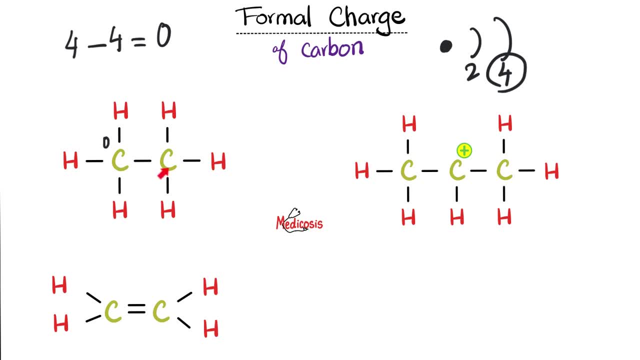 neutral and has a formal charge of zero. how about this carbon? same story: one, two, three, four. i expected four, i found four, so zero. it's also neutral. now let's look at this carbon. carbon is still carbon, which means i still expect four valence electrons, which means i expect four. 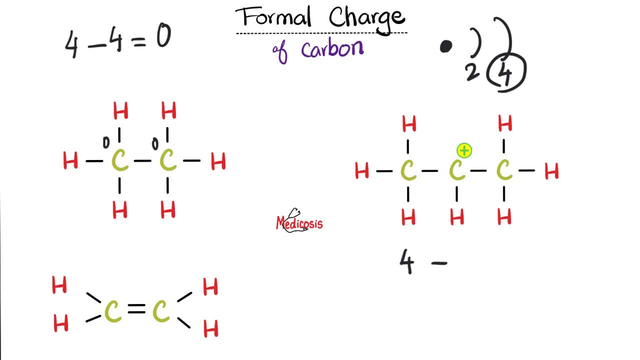 four valence electrons. okay, how many bonds do we have here? i have one, two and three. four minus three is positive one. so the formal charge here is plus one. let's try this: carbon. how many bonds or how many valence electrons do i expect? four, how about here? one, two, three, four, four minus four? 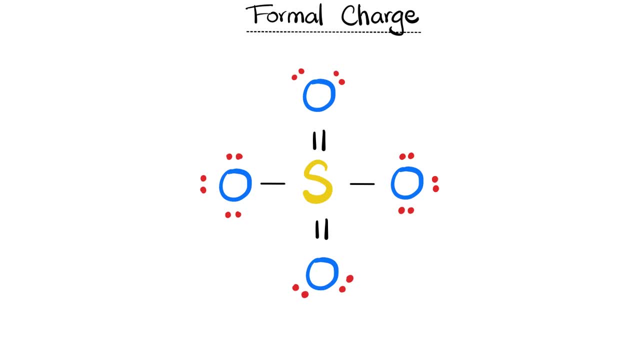 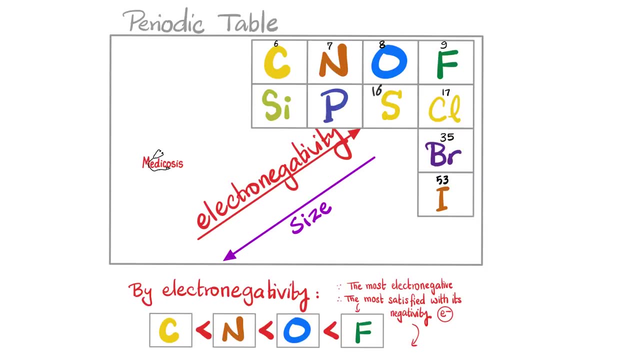 equals zero. this is neutral. now can you find the formal charge for this molecule as a whole, whole spelled w-h-o-l-e. first look at the periodic table. is this a clock or is this a given, a problem table? i expect oxygen to have what? eight electrons, so two in the first shell and six electrons in the. 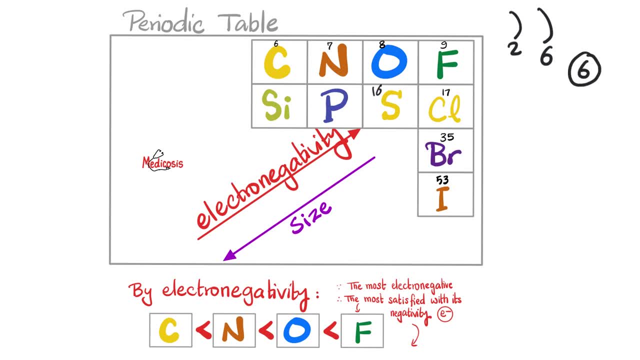 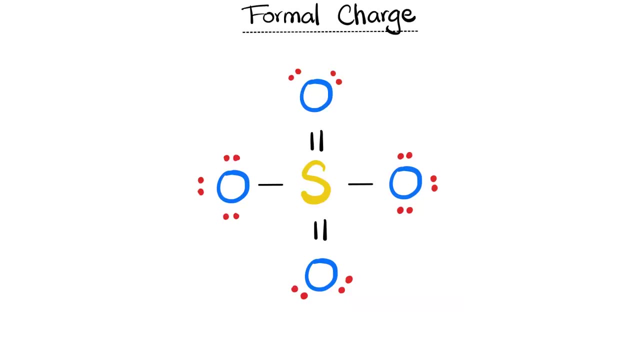 valence shell. i expect six. that's what i expect from oxygen. amazing, how about sulfur? sulfur has 16 electrons, two in the first shell, then eight, that's 10. 10 plus 6 is 16. okie dokie, i expect mr sulfur to have six as well. now let's try this. look at this oxygen. i expected six valence. 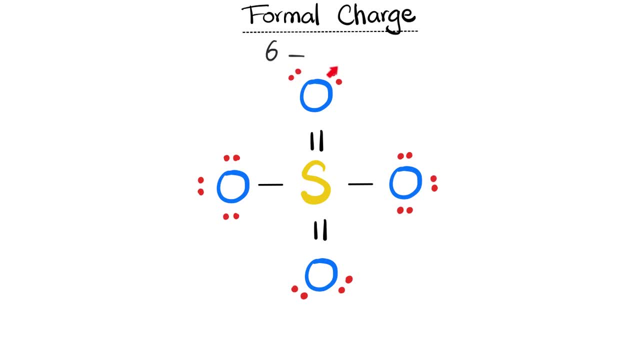 electrons. how many did i see? actually one, two, three, four, five and six. six minus six equals zero. this oxygen does not have any charges. let's look at this one. i expect six, because it's an oxygen. how many did i actually see? one, two, three, four, five, six, seven. six minus seven is negative one. 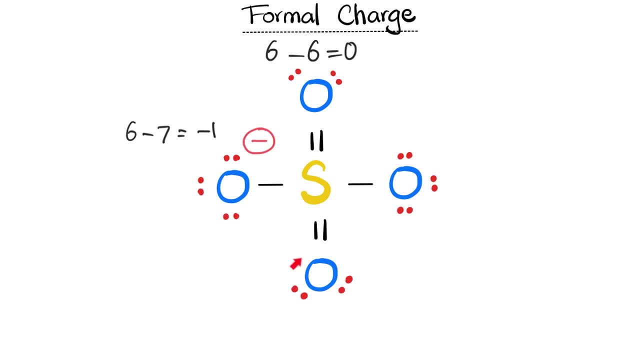 so this oxygen has a charge of negative one. how about this oxygen? i expected six, i found one, two, three, four, five and six. six minus six is zero. as for this oxygen, i expected six, i found one, two, three, four, five, six, seven. so six minus seven is negative one. so this oxygen has a formal charge of negative one. 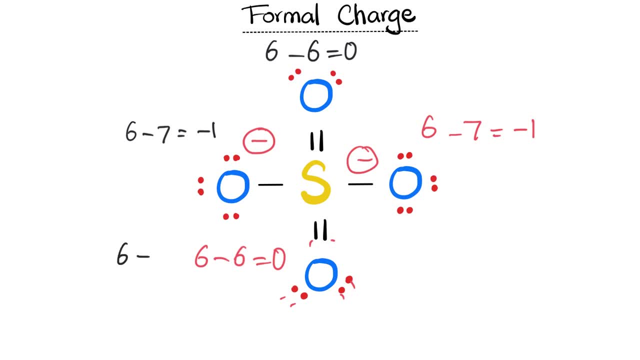 how about the sulfur? i expected six and i found one, two, three, four, five, six, six minus six for the sulfur gives me zero. so in total there is a formal negative one charge here and negative one. that's why the formal charge for the entire molecule is negative two, and that's why you write. 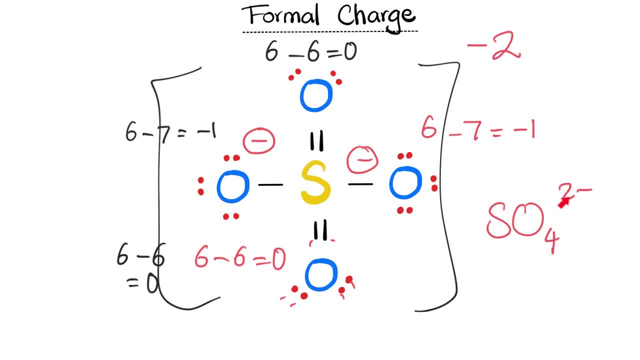 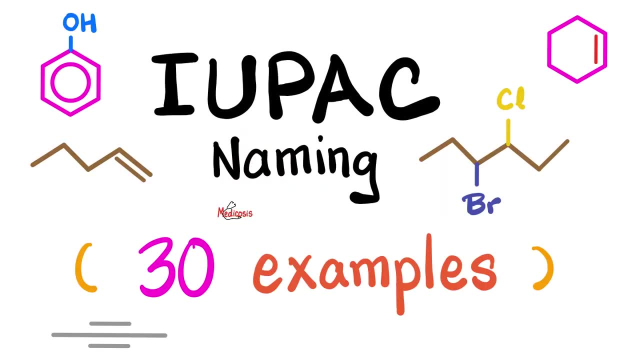 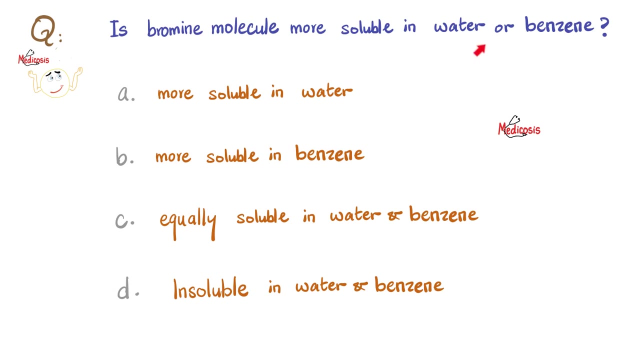 s o four. two minus like this. this is where the two minus came from, one here and one there. you do not want to miss the next video in this organic chemistry playlist where we'll talk about the iopec systematic naming quiz time. is bromine molecule more soluble in water or more soluble?